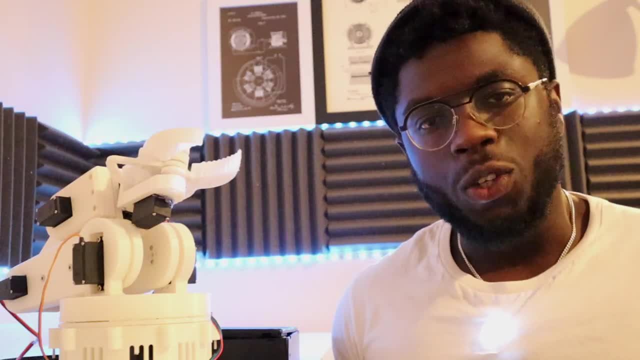 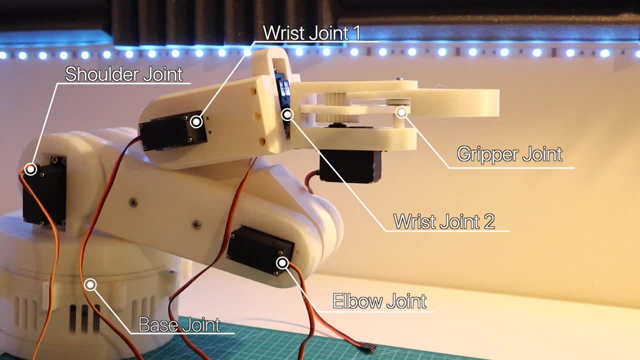 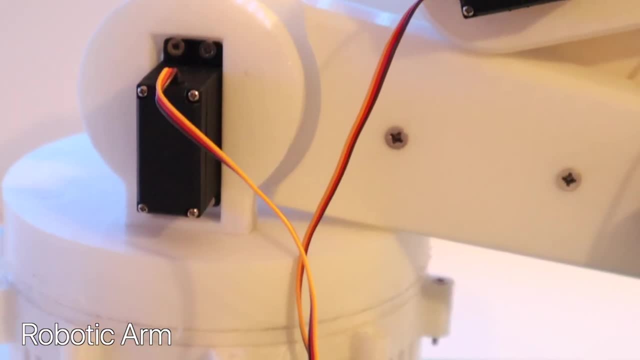 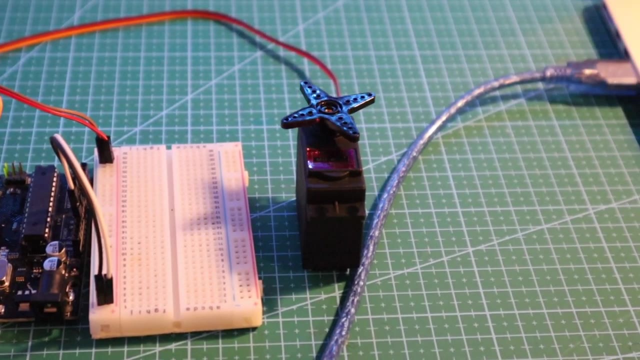 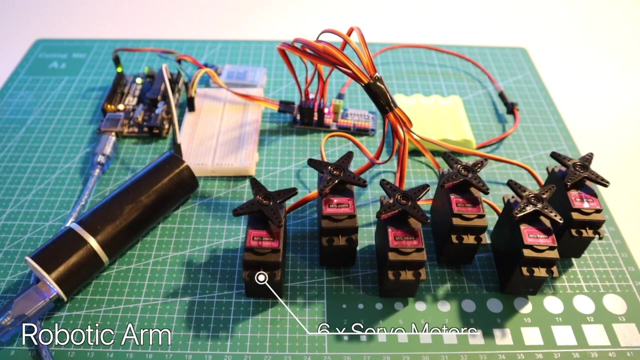 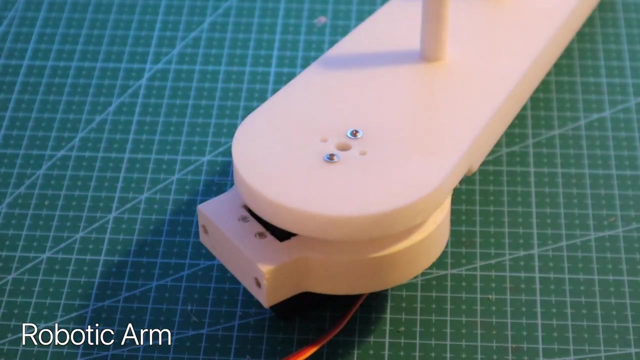 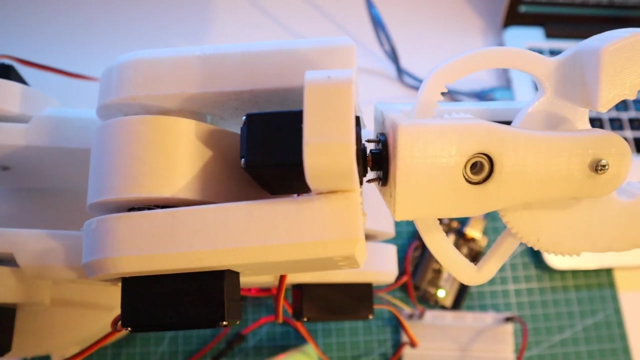 wireless and portable. this means we can have a more natural interaction when controlling the robot. And since it's weirdly all Mirko And then we can assemble each server motor into a 3D printed robotic arm And program it. And this is pretty much what we'll be building. 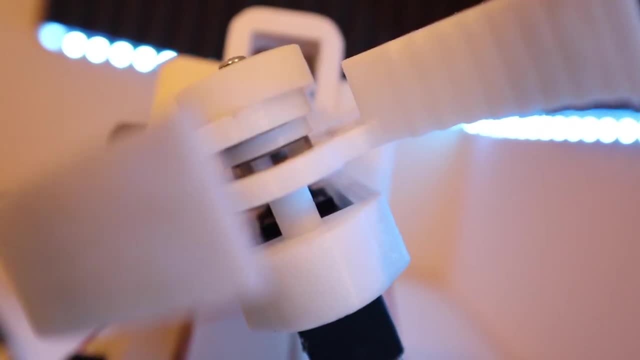 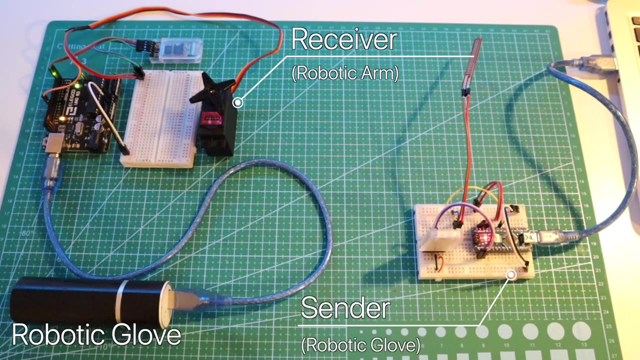 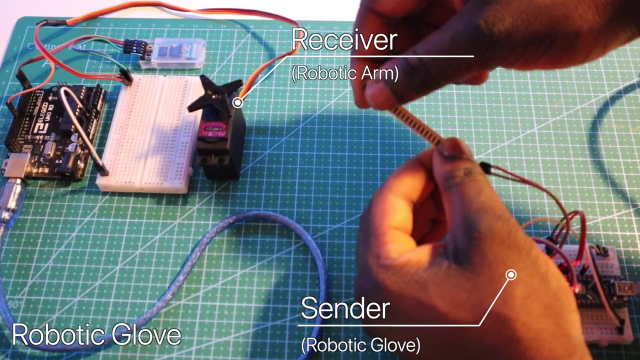 But the question is, how do we communicate with the robotic arm Using hand gestures from the glove? So, when it's all stripped down, we've pretty much got a sender and a receiver And we're using a sensor to send values to the robotic arm to move the servos. 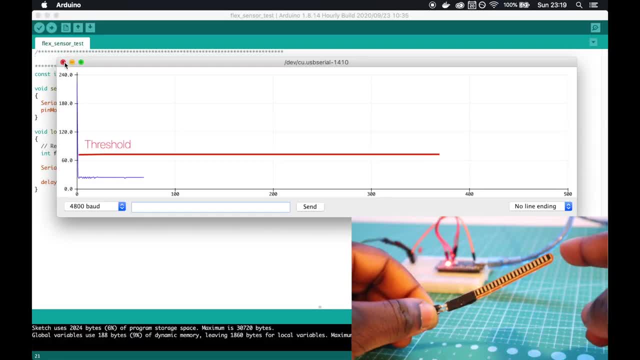 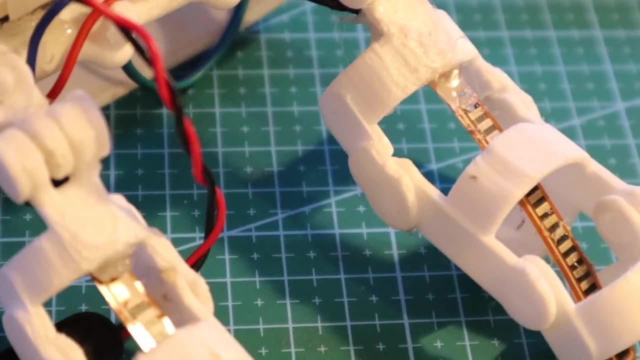 And this is done over Bluetooth. So, having a closer look, when we bend the sensor, the value changes. Now if we exceed a specific value, we can send a message over the Bluetooth to turn that specific servo motor. So in that case, when we bend our finger, we can in turn control the robot. 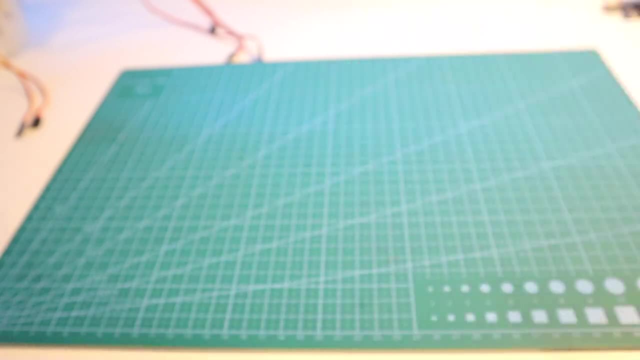 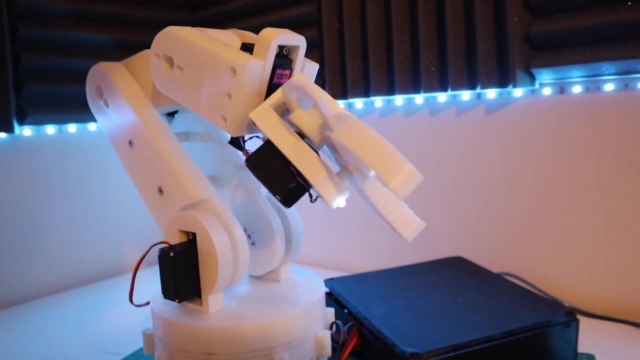 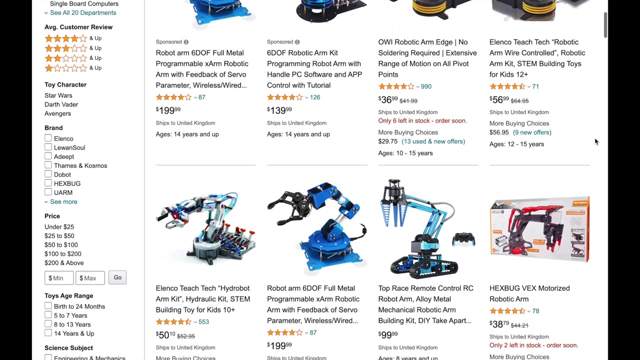 We're also going to cover how the 3D arm is printed and adding more flex sensors to make a complete robotic glove later on. But let's get back to the robot and let's get started. Assembly of parts, The robotic arm. Now there's different examples of robotic arms online. 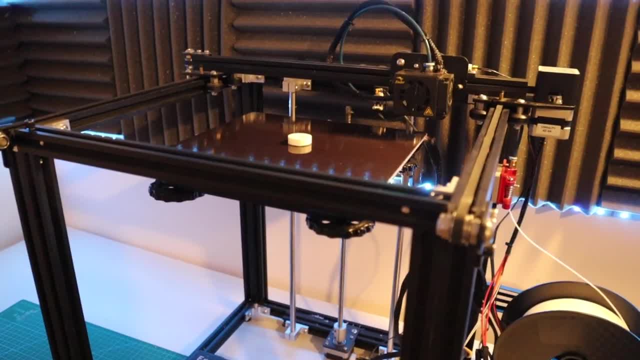 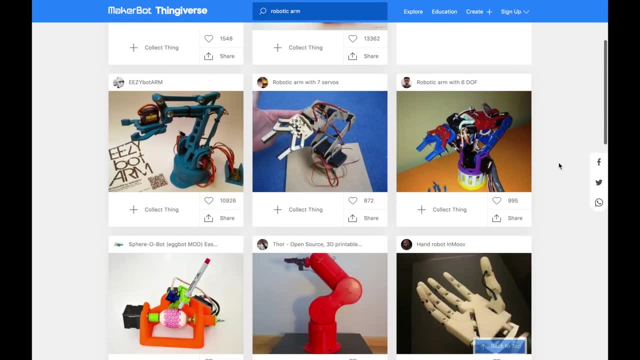 You can either buy one or 3D print one, But since I'll make another version, this one was 3D printed and if you've got a 3D printer, There's only good examples of free robotic arms to build. This is the one I'll model mine after. 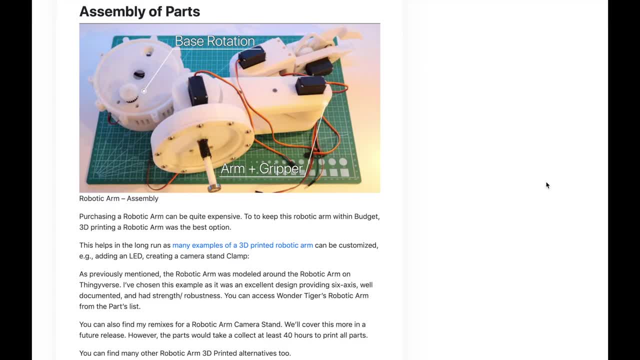 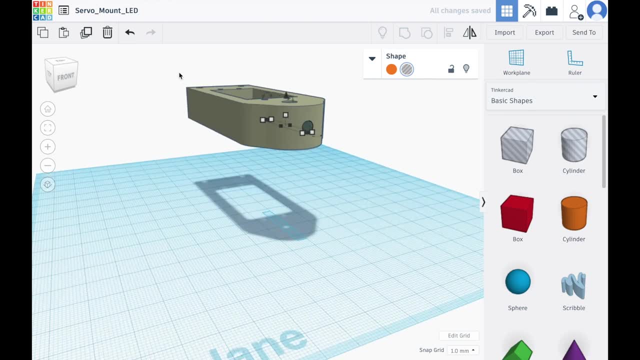 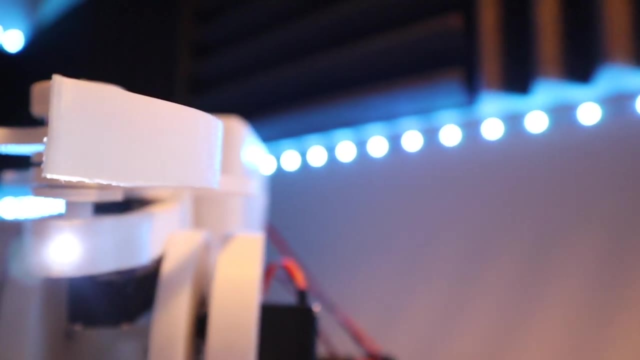 And credit goes to this maker And you can find more instructions on the assembly on the article in the description below. So this robotic arm was slightly modified so we can add a hole for an LED for the gripper part of the motor. Now 3D printing the robotic arm was pretty long. 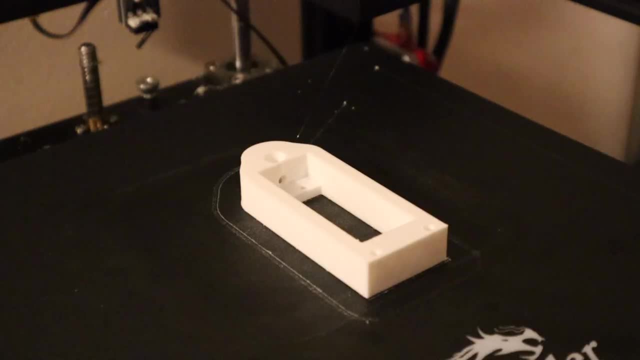 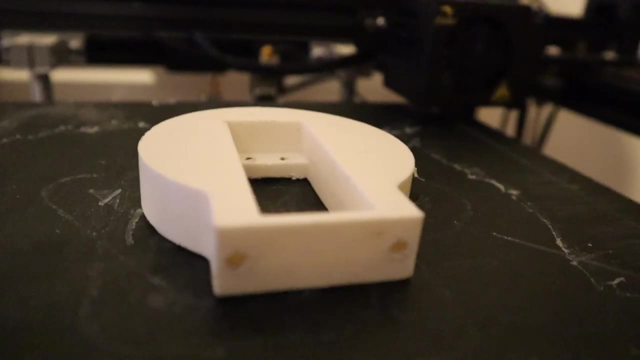 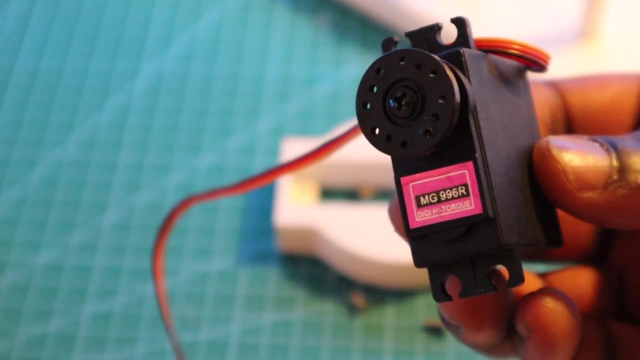 And, if you want, you can get an out of the box robotic arm instead. But taking the 3D printing approach helps create custom parts like this And we can print the other parts. Now that they're all printed, we can now assemble it all together with the server motors. 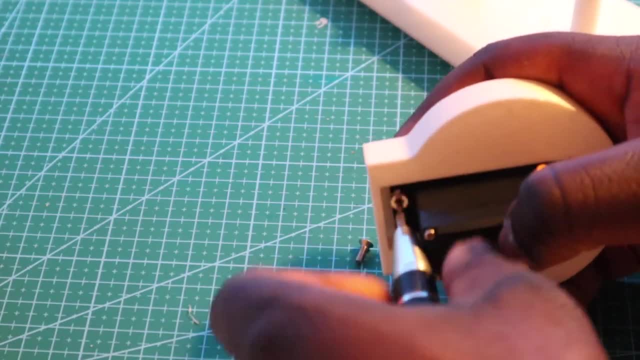 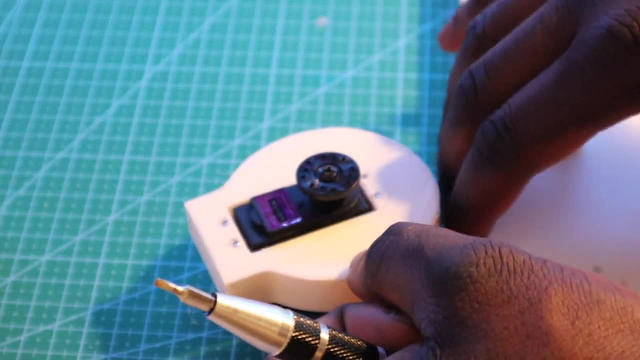 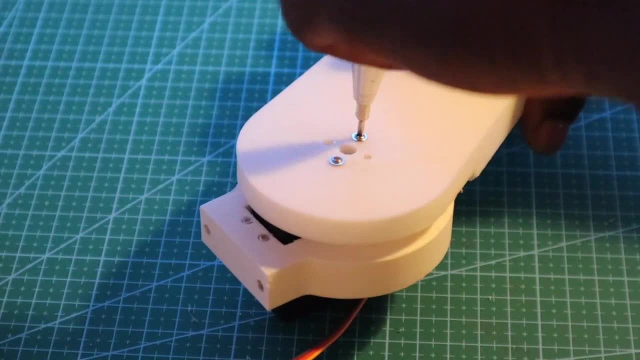 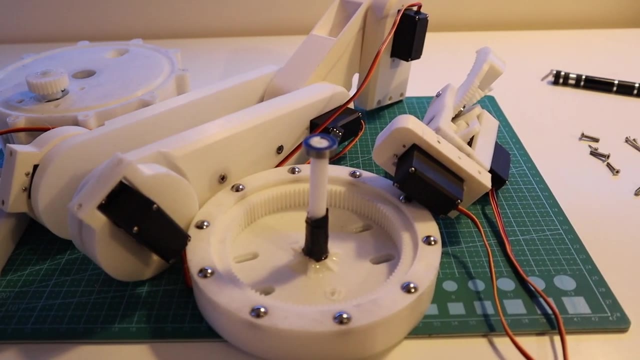 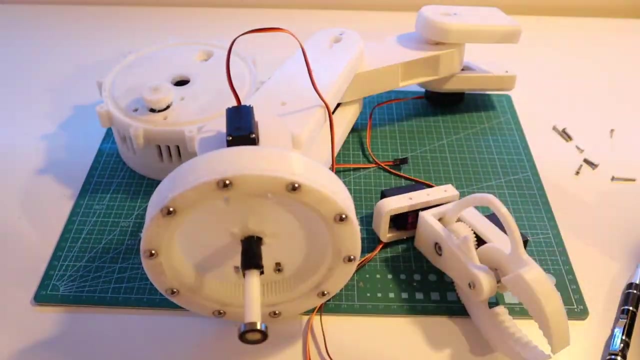 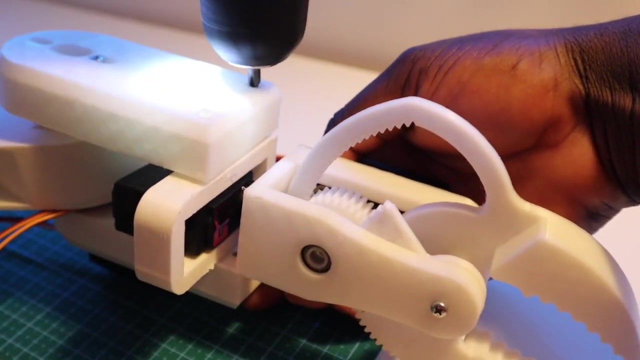 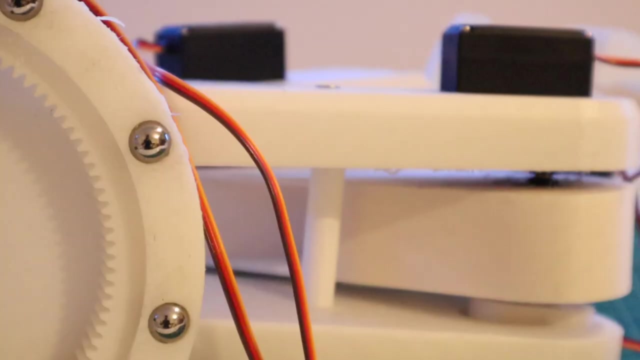 robotic arm build. And these are the parts that make up the robotic arm once we fully assemble it- And here we're just assembling the gripper part- slash claw to the stem of the robotic arm. Now, the good thing about the robotic arm is that it has ball bearings, so we can smoothly 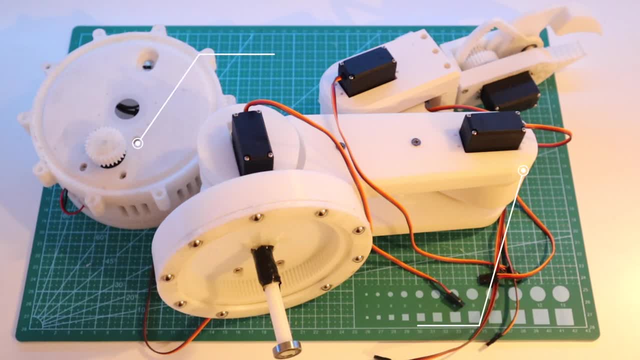 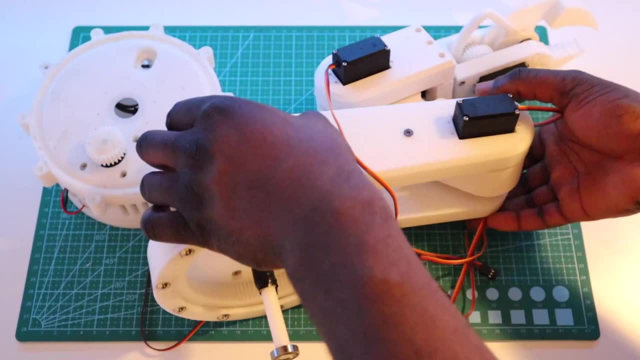 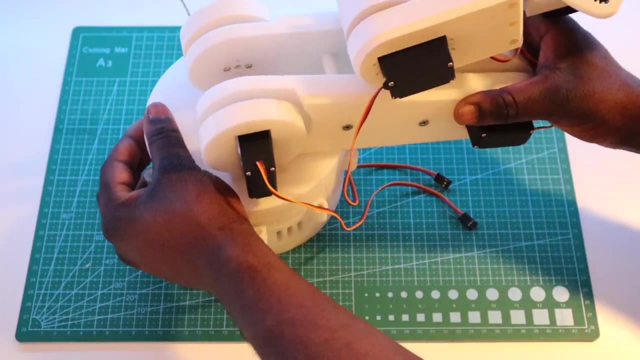 rotate left or right. The two main parts are the base rotation and the robotic arm itself, And now that we almost assemble it, all we need to do is insert these two together and lock it in place, And that's it for the assembly. 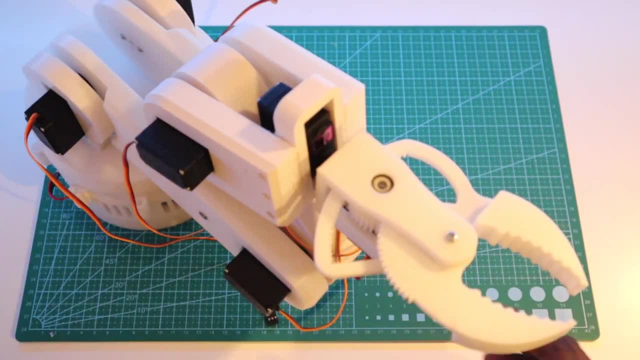 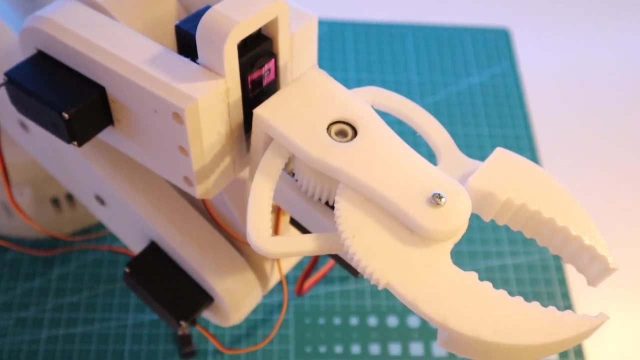 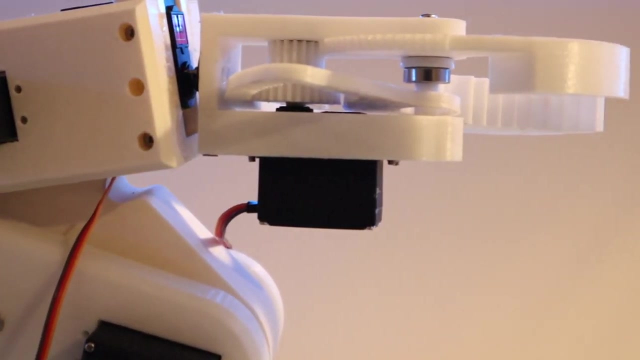 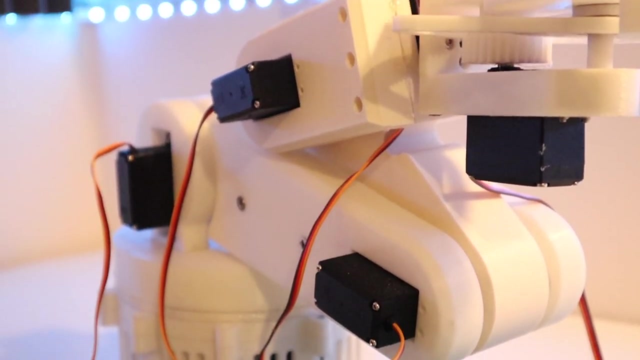 Thanks for watching. Each of the 6 server motors have now been mounted in place And each of these motors can now be programmed to move or perform a task like picking an object. If you've got any other ideas, let me know in the comments below. 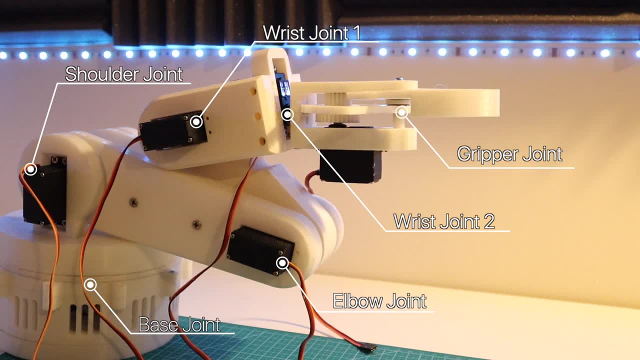 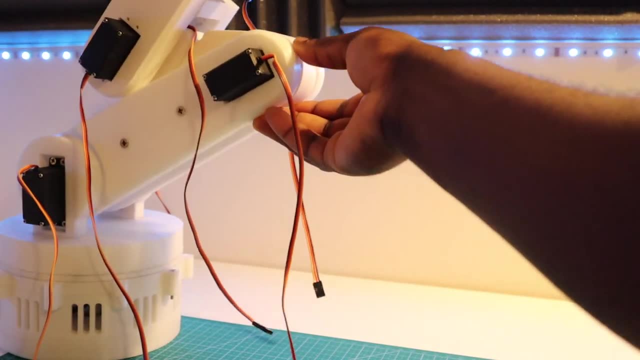 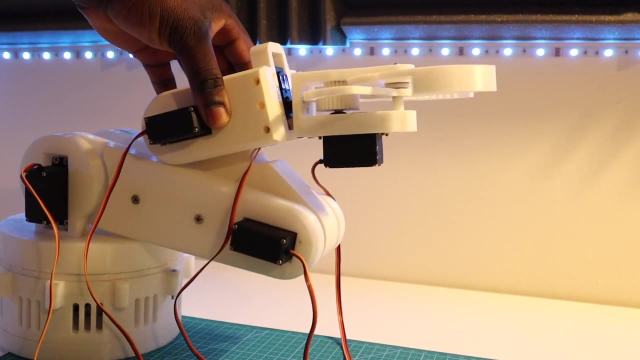 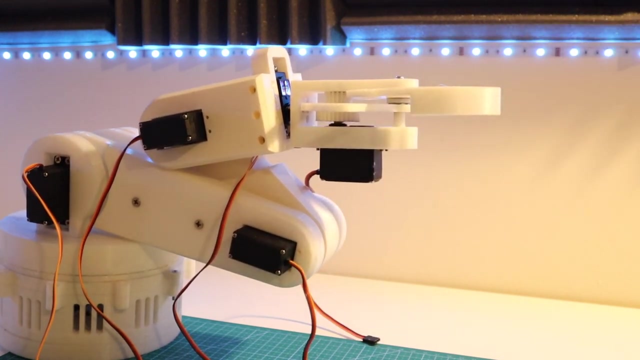 Now the robotic arm is assembled, We can see the individual parts. These motors play in the rotation and movement of the robotic arm. For example, we can rotate the shoulder joint as well as extending the elbow joint, And we can even rotate the wrist joint, which will be the claw. 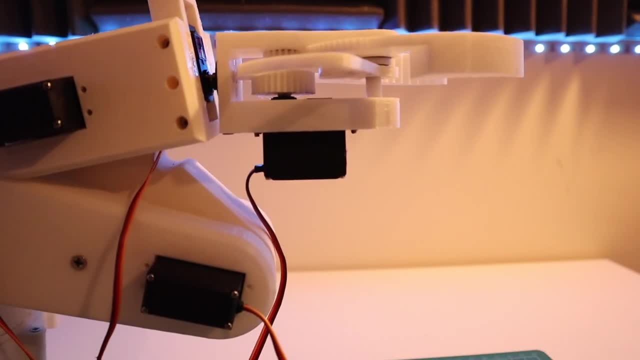 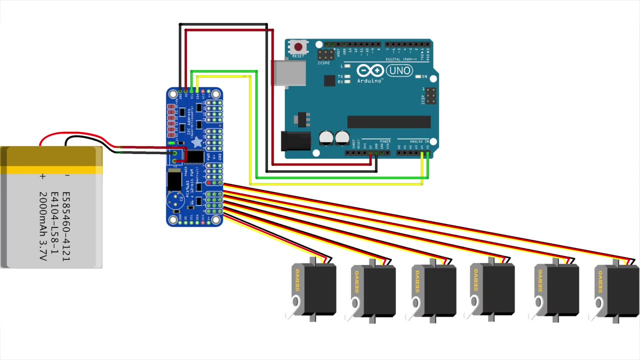 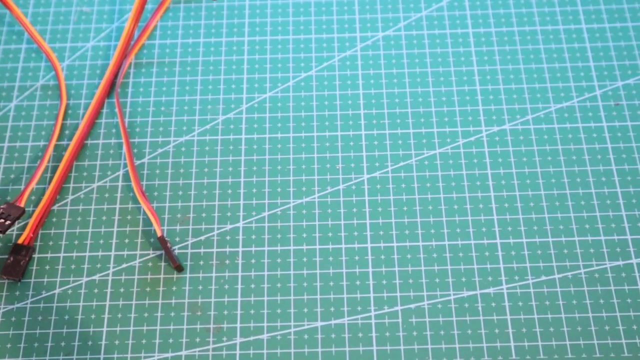 Server motor wiring Introducing the Arduino. Now we have the server motors all assembled into the robot. We can now start the assembly All assembled into the robotic arm. We'll still need to somehow power the server motors. In order to power each individual server motor, we'll need a driver, and this is where the 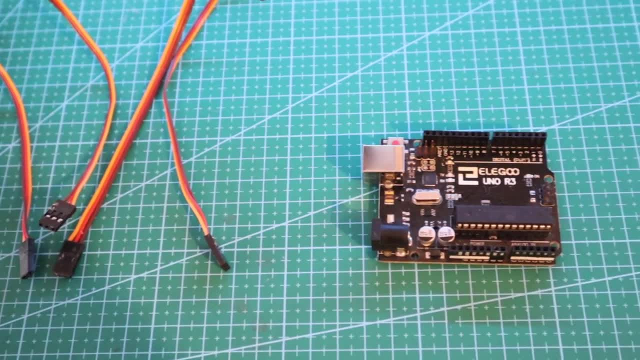 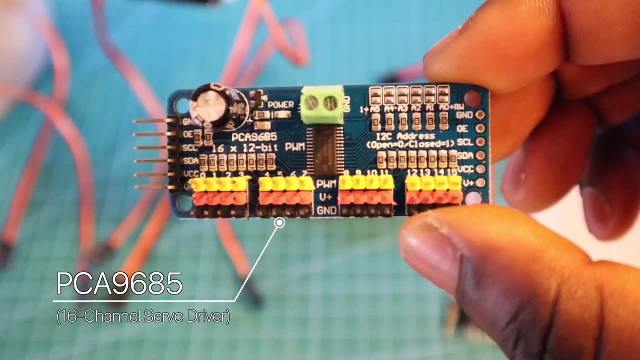 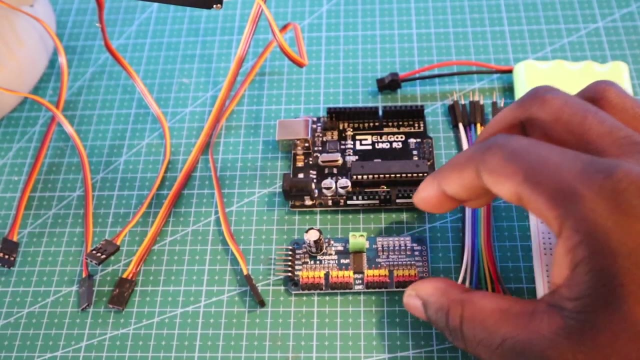 Arduino comes into the picture. Now. Arduino's are open source, so there's different copies. We'll be also using the server driver, and the server driver we'll be using to do this is the PCA 9685.. PCA 9685.. much what we'll need to power the six server motors, which include jumper. 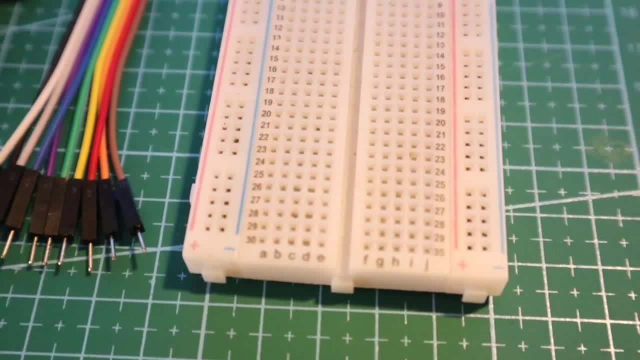 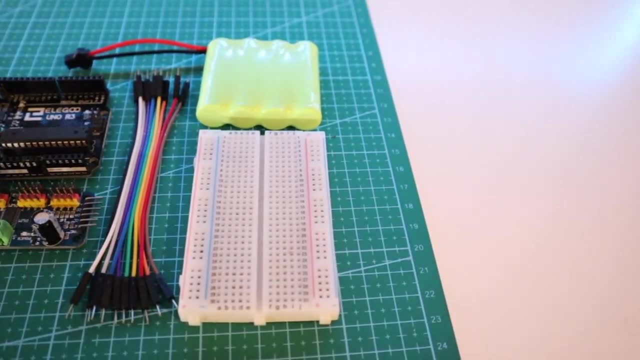 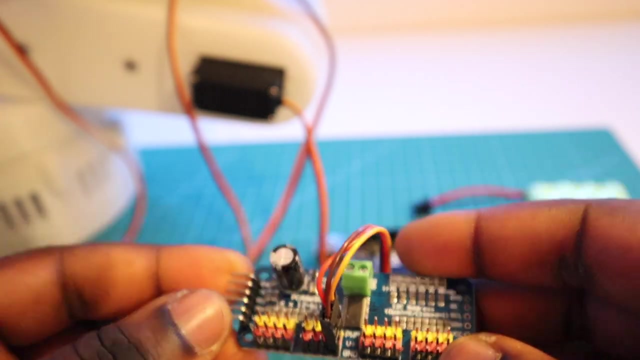 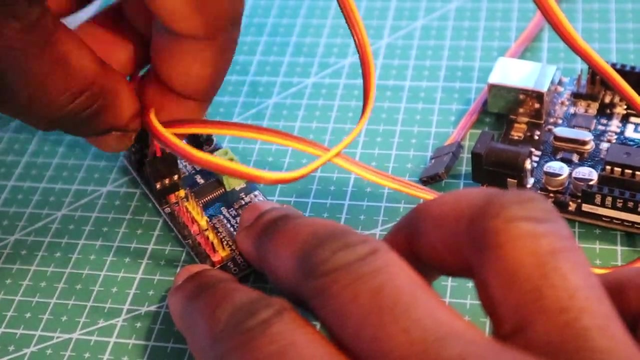 wires, a breadboard and a 5 volt RC battery pack. Now we can slowly assemble these all together. Now attaching the server motors is as simple as plugging them in into their color coded pins. Now we can add the other five in and all of these all attach to the individual motors of the 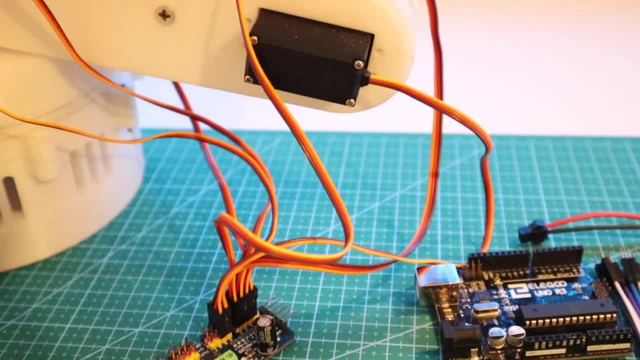 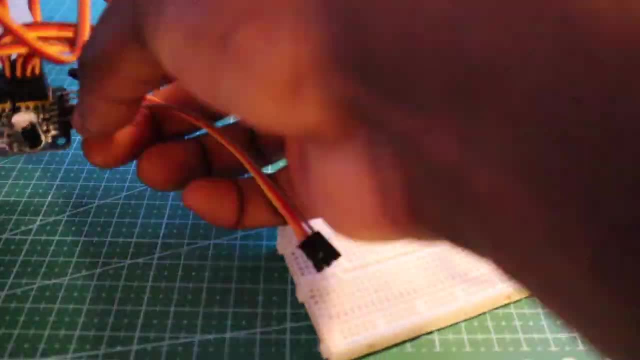 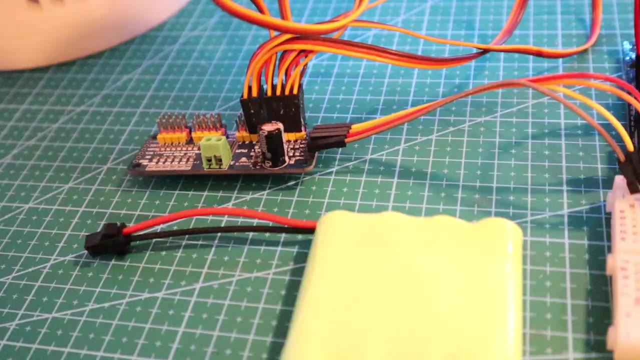 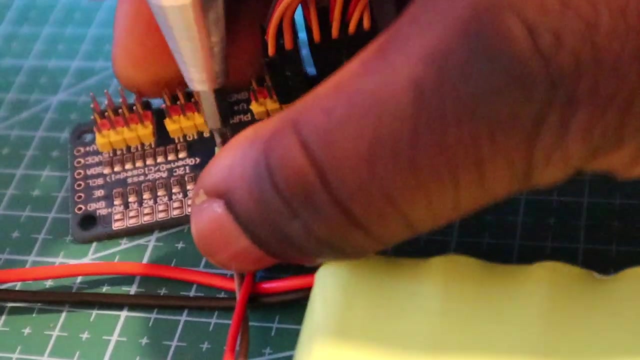 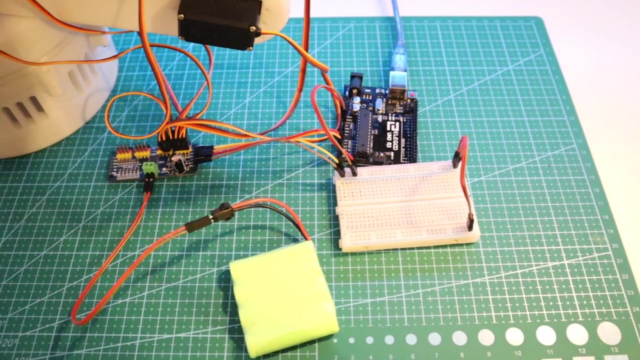 robotic arm which can drive any individual server motor on the arm. We can pretty much wire them all together based on the diagram provided. Now we can add the 5 volt RC battery pack to the server driver to power the the server motors, And we can do this by screwing these in. 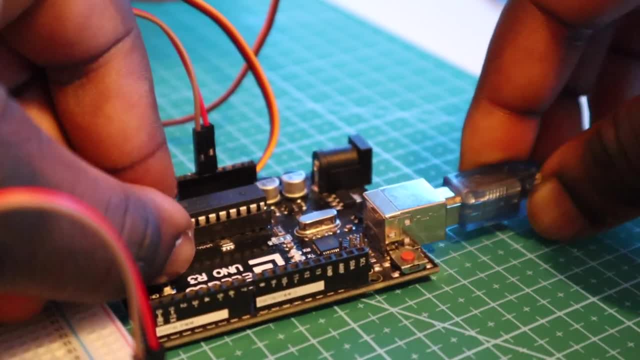 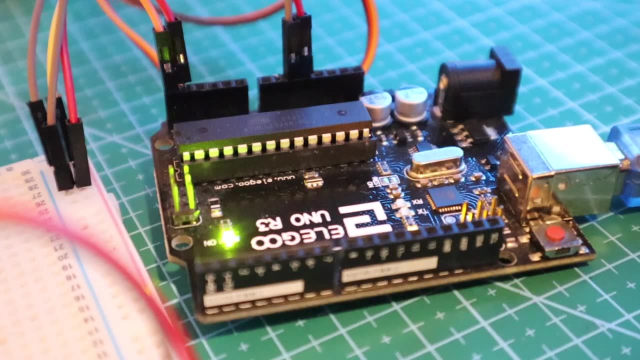 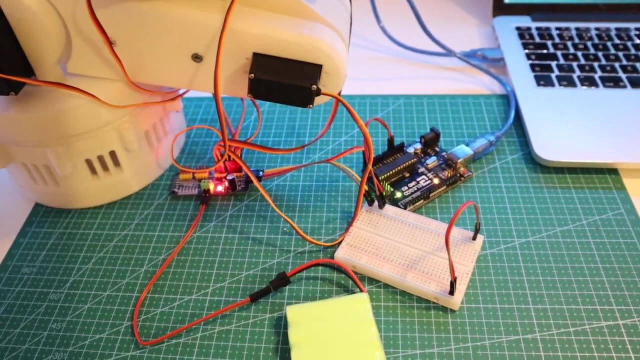 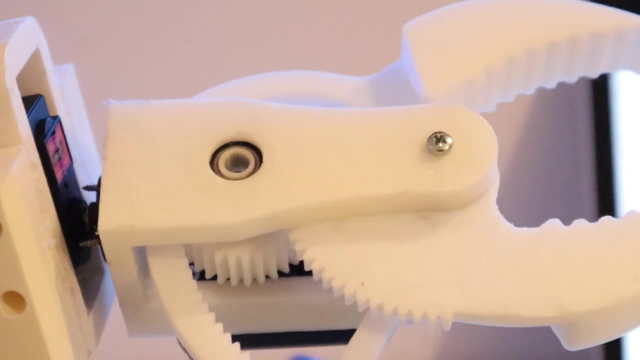 We can now hook up the Arduino to our laptop and load the code to power the server motors, And you can find all the codes in the description with each test code. In this example we're just testing the server motors for the claw slash gripper. 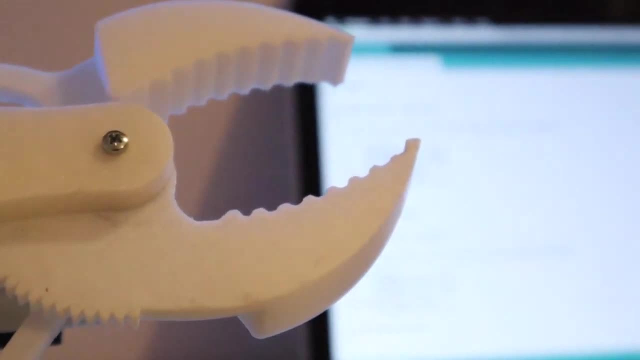 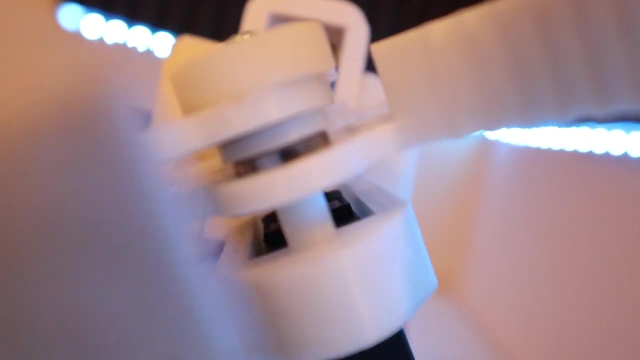 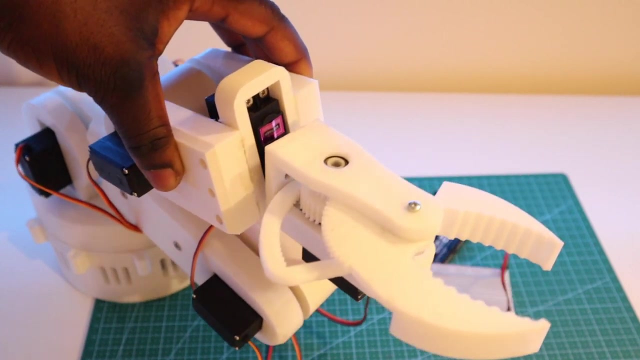 Now we have the six server motors working, we have one more thing to do. We still need to figure out a way to make the robotic arm rotate left or right. Now the robotic arm is gaining a bit of weight and using the standard server motor isn't. 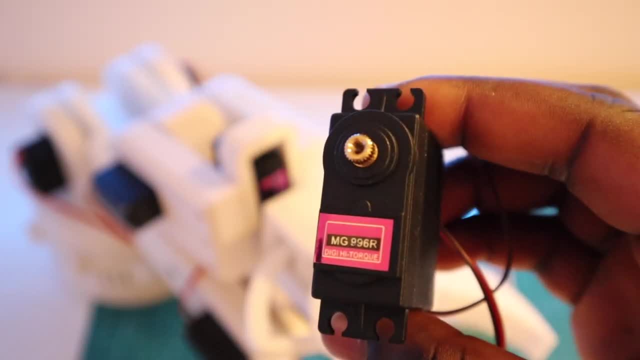 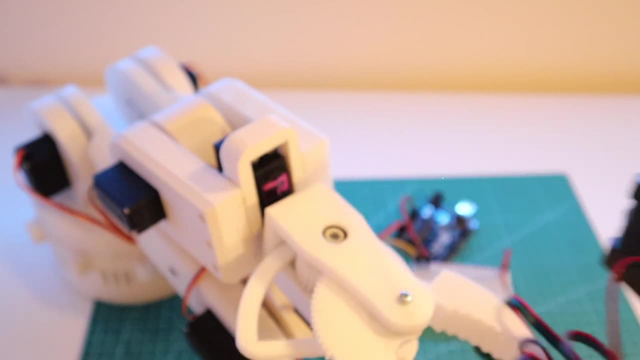 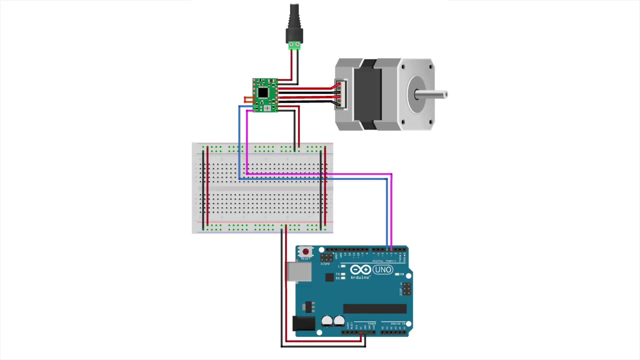 powerful enough to move it. So instead of using a standard server motor, we're going to use a stepper motor, which is pretty accurate as we can control the number of steps- slash rotations needed. Now this is the diagram that shows the setup using the stepper motor and the driver. 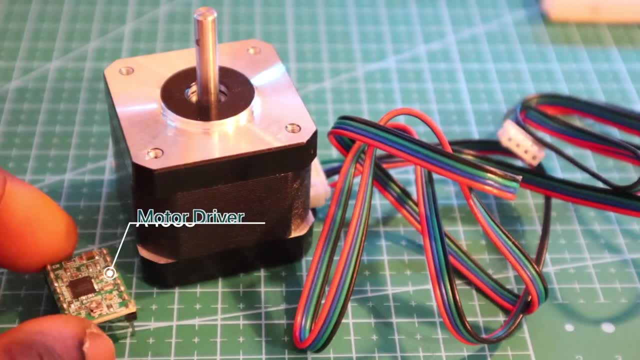 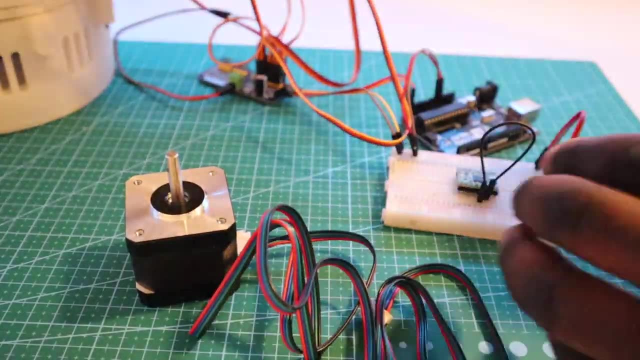 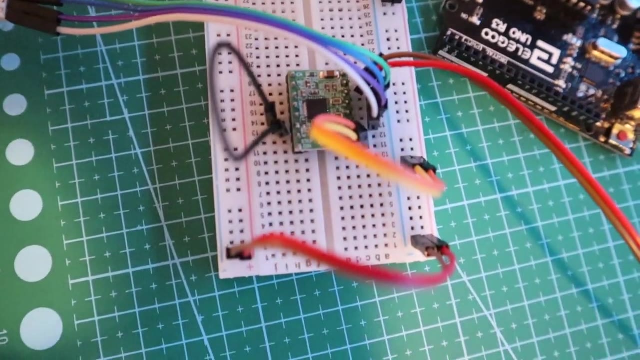 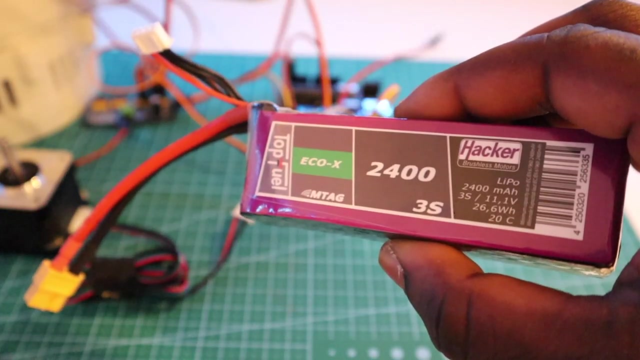 The stepper motor comes with its own driver, being the A4988 driver. Now, based on the diagram, we're just going to assemble it all together. The stepper motor requires a higher voltage compared to a server motor, so we're going to use an 11.1V LiPo battery to supply the power. 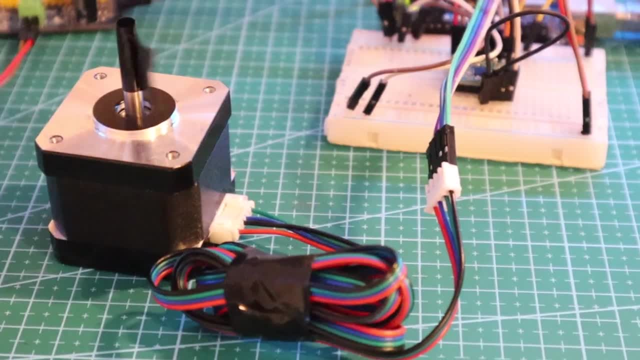 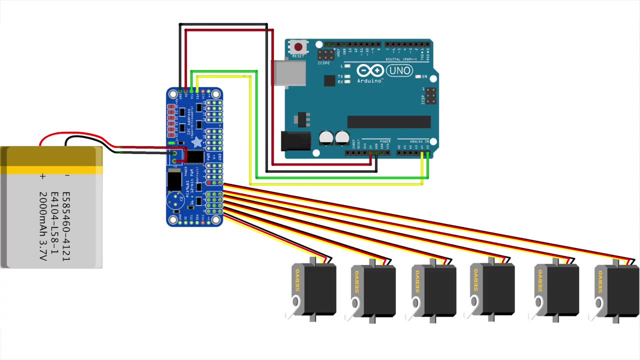 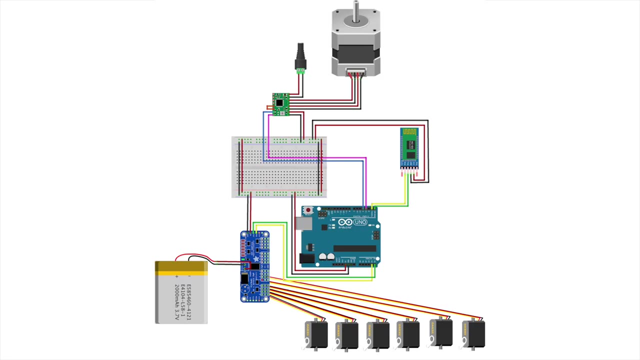 And loading the test code, we can see it rotate clockwise. We can even smoothen the stepper motor movements by adding a capacitor. So an overview. We went from adding the six server motors to adding the stepper motor And now this is the full robotic arm electronic diagram. 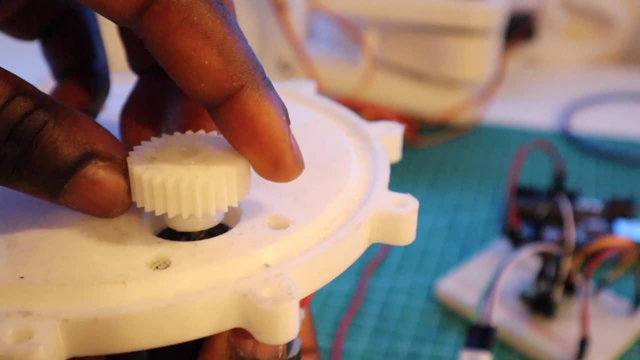 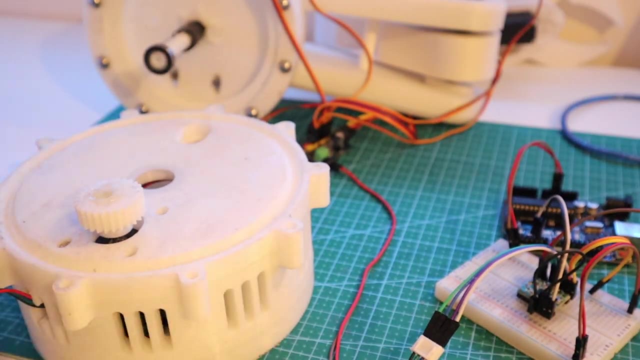 And now we're happy with it. we can mount the stepper motor into the base of the robotic arm Which we can line up and eventually screw in. The stepper motor will be mounted to a gear tooth, which would in turn allow the stepper 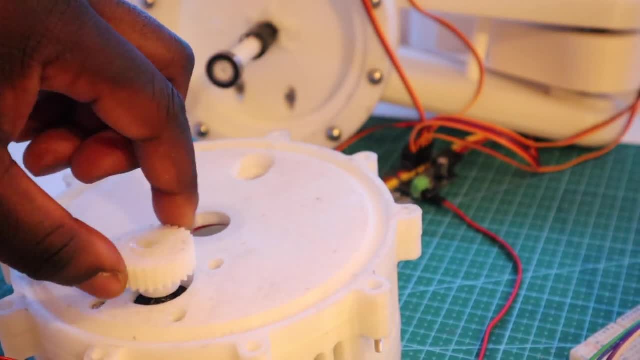 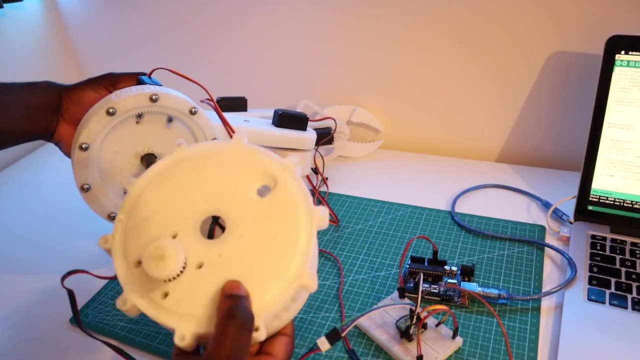 motor to be mounted to the base of the robotic arm. The stepper motor will be mounted to a gear tooth, which would, in turn, allow the stepper motor to be mounted to the base of the robotic arm And, as you can see, we've got the smaller gear tooth and the larger one in the back. 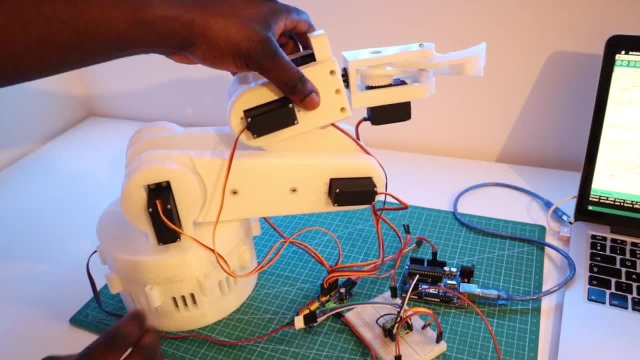 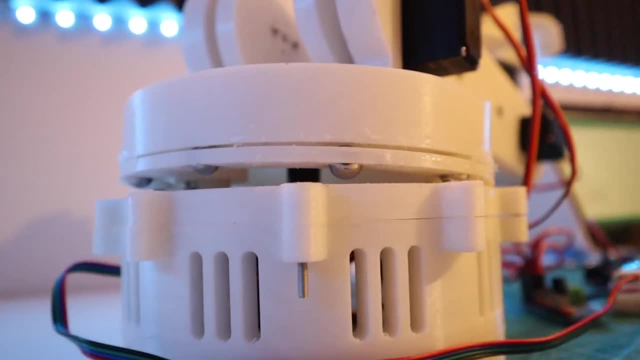 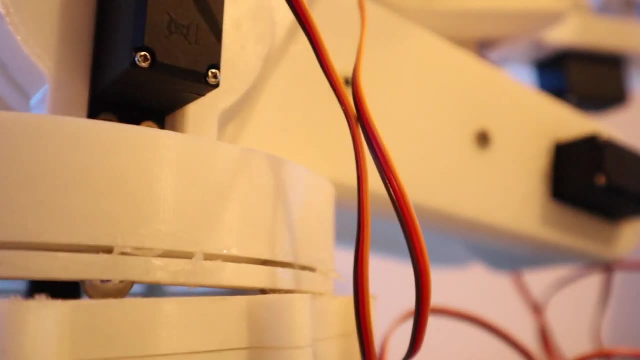 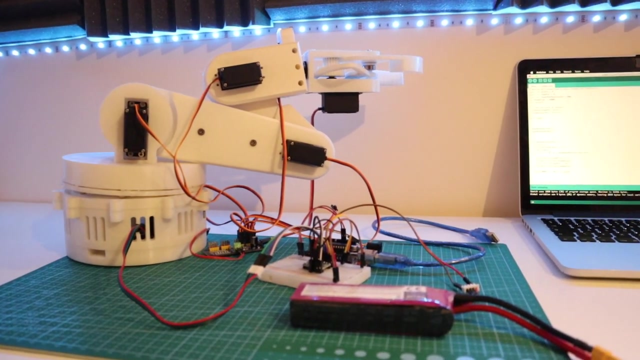 And we can place these two in and they're locked in place. You can also see that the ball bearings provide for a smoother contact, also reducing the noise. And now we've got the robotic arm all assembled, we can load in the test code to rotate the. 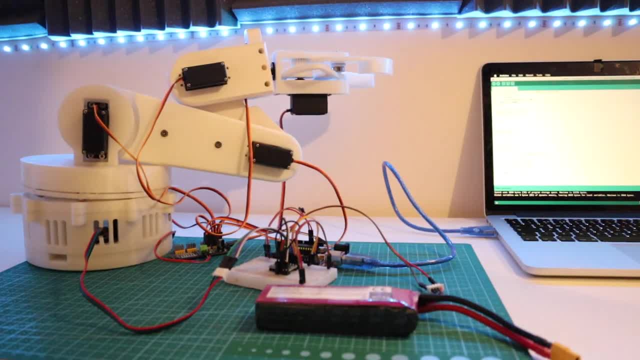 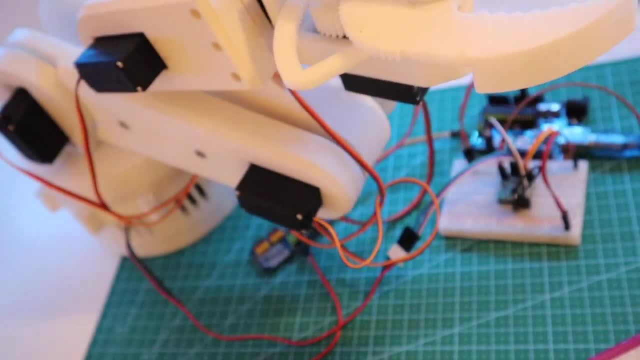 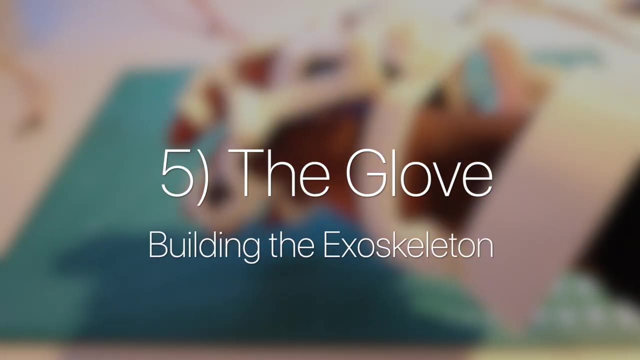 robotic arm. And that's pretty much it for the robotic arm, And if it's the robotic arm you wanted to do, you can pretty much stop here. The next part will be on how the glove is assembled. Assembly of parts. the robotic glove. 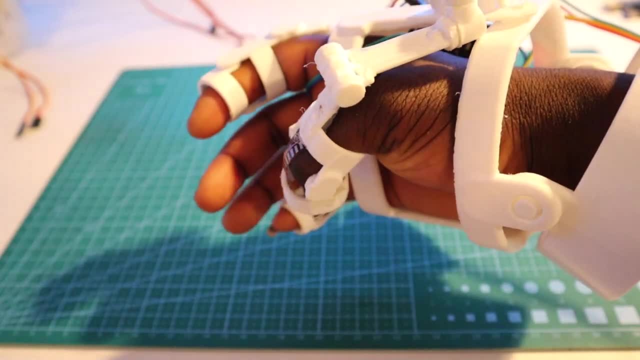 Now staying true to the aesthetics: The robotic glove is the most important part. The robotic glove is the most important part. The robotic glove is the most important part. The robotic glove was also 3D printed, but you can use a standard glove to work with. 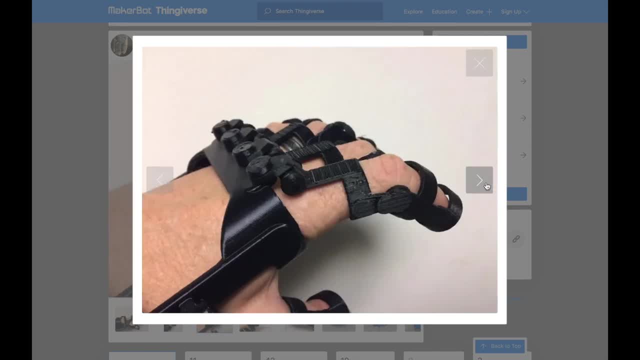 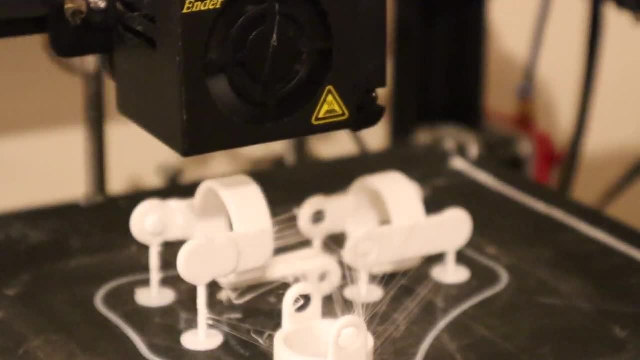 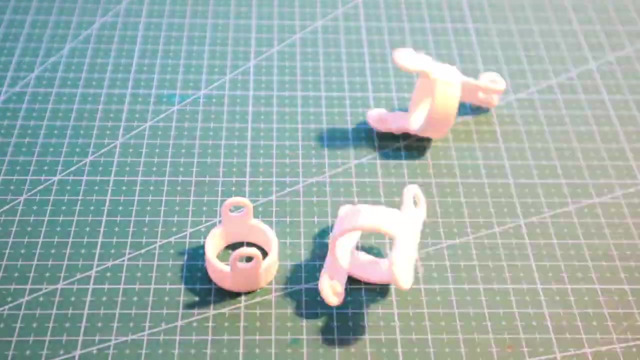 which I used with earlier versions. Now the glove comes in parts which can be printed off individually. In this example I'm printing off the index finger of the robotic glove, which comes in three segments. The three parts representing the finger joints can all be snapped in and, once all assembled, 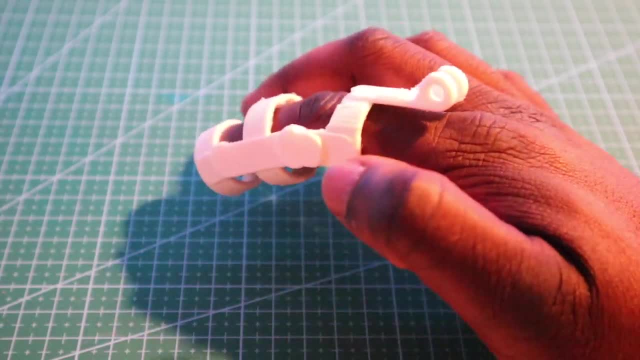 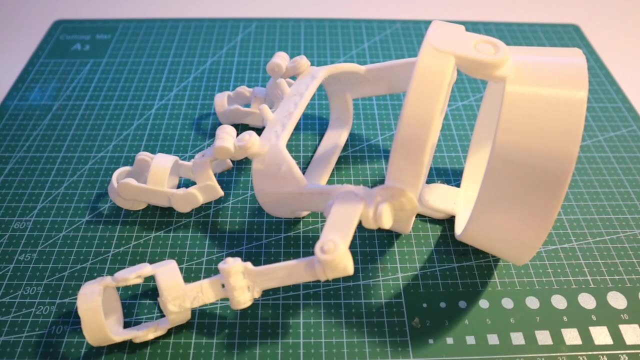 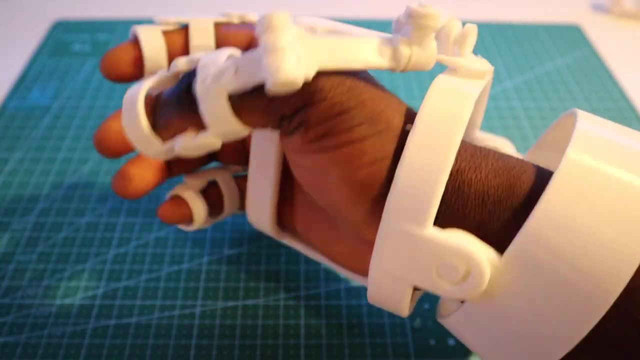 it fits perfectly on my robotic arm. And there we have it. that's the finger joint, And this is how it looks when it's all assembled. Now the glove provides a good degree of freedom, which is a bonus. So now that's done, let's find out how the robotic glove's sensors work. 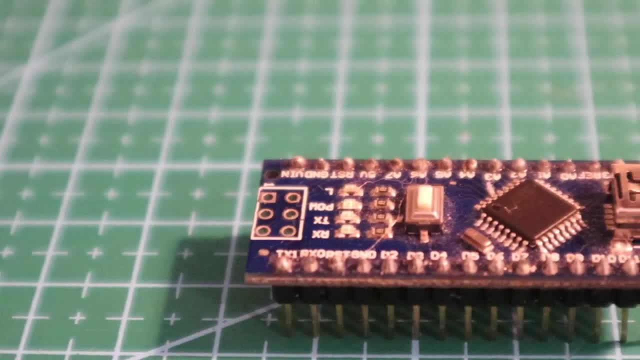 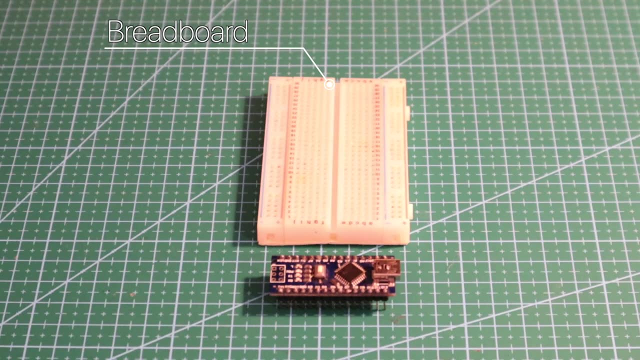 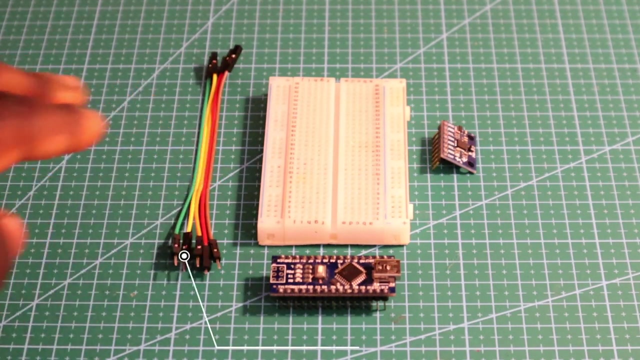 And from the part list, we'll need an Arduino Nano. This will be ideal, since it's small enough to fit on our hand. Also a breadboard for prototyping And an accelerometer to measure the changes in the hand movement, And some jumper wires. 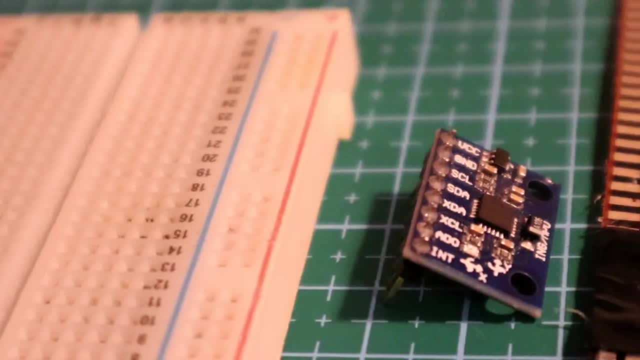 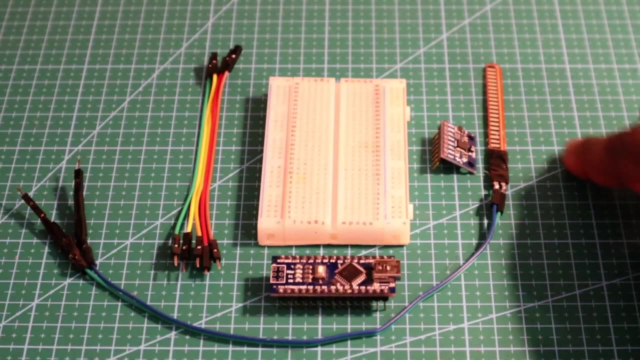 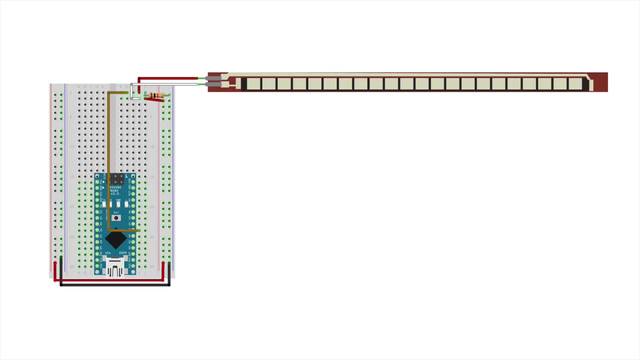 And the flex sensor- These two types of sensors would be the main focus- And lastly, a 10 kilo ohm resistor for the flex sensor. To start off, the following wiring would be required: The following wiring would focus on the flex sensors, with the output of the flex sensor. 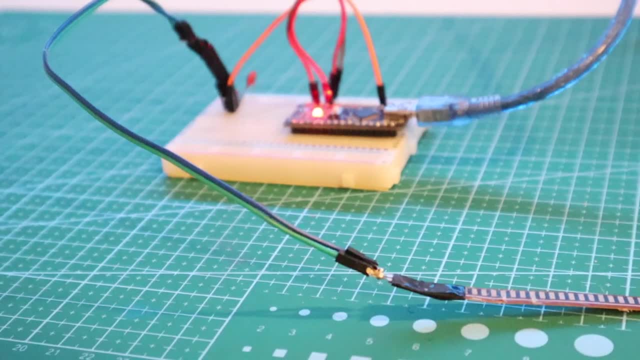 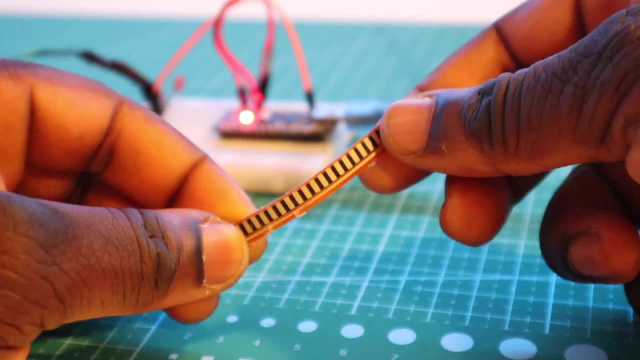 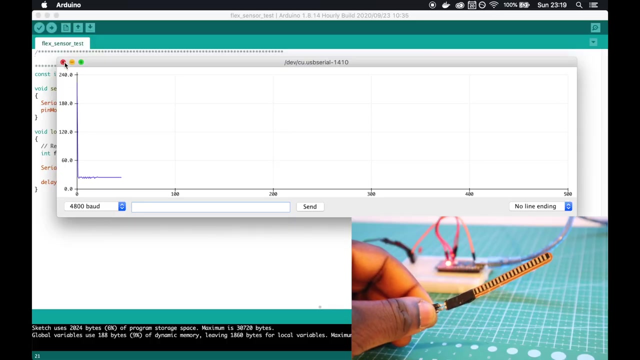 going to analog 3, on the Arduino, And once that's wired up and the code has been uploaded, which you can find in the description, we can test it out. Now the flex sensor works a bit like a potential divider, And as the flex sensor bends, the resistance changes. 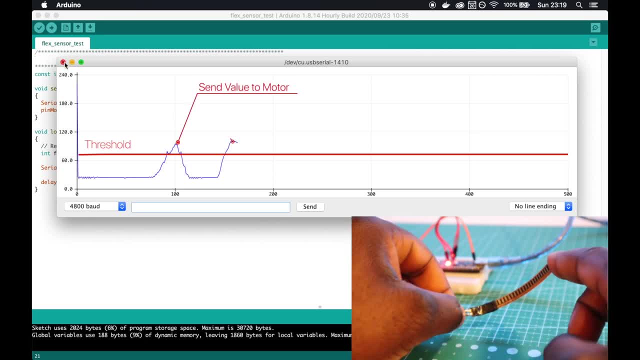 And here's a graphical look of the flex sensor value changing. Now, put in a threshold at, let's say, 70.. And here's a graphical look of the flex sensor value changing. If it passes this, we'll send a value to the robotic arm's Arduino through Bluetooth. 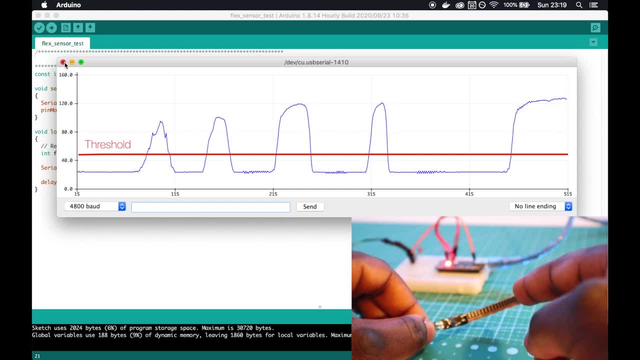 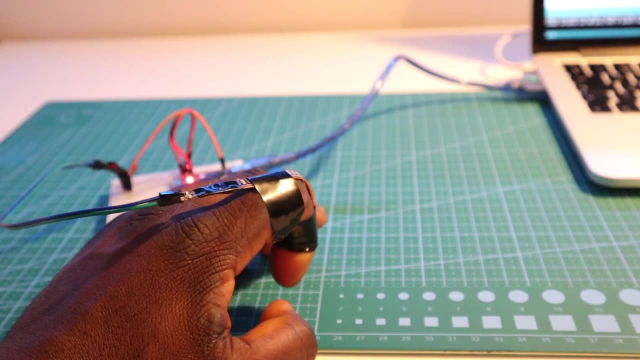 And by holding the flex in place, we can also hold the position of the servo motor And, in turn, the robot. And by taking this idea and attaching it to our finger, there we have it. We have a sensor that can detect the changes in our finger movement. 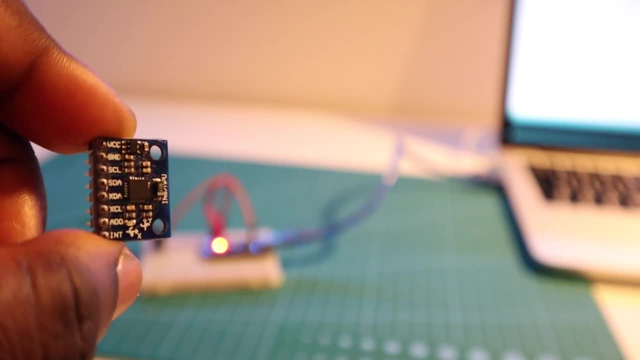 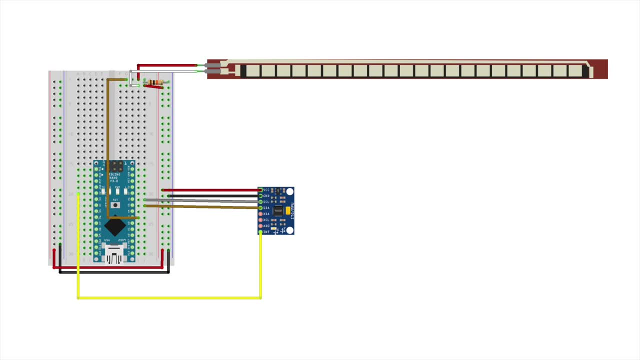 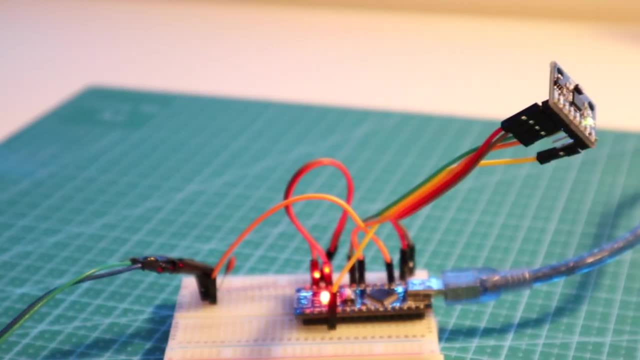 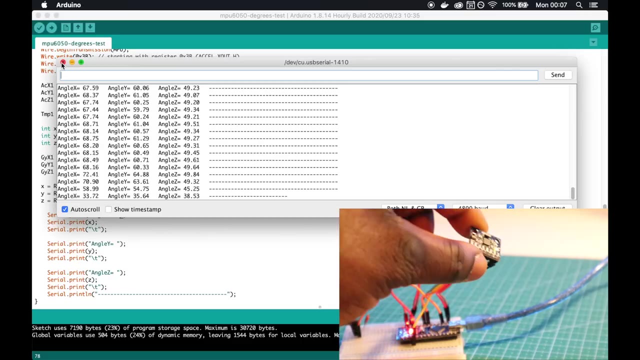 And here's a graphical look of the flex sensor value changing. We have these changes in our hand movement And this is the diagram with the updated accelerometer in place And now we can upload the accelerometer test code And by moving it slightly, we can see how the x and y coordinates change based on the. 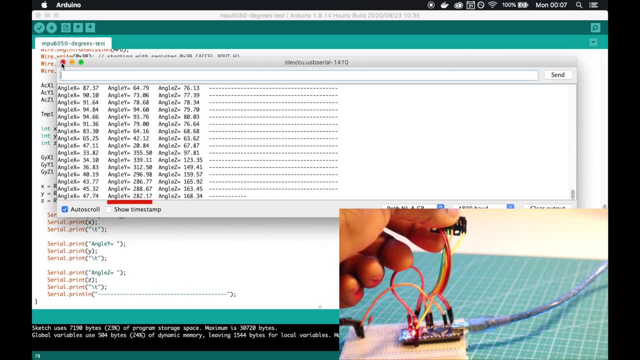 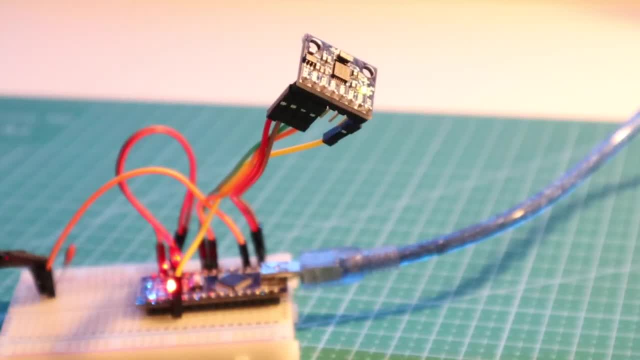 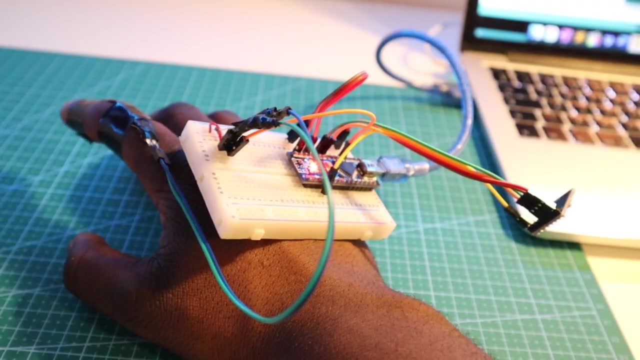 relative position of the accelerometer moving left to right, up and down. Stereo Accelerometer Testung. Stereo Accelerometer Testum. Stereo Accelerometer Test人. pretty much it what we'll need and how it's assembled. With the two sensors alone, we can control the robotic arms gripper to open and close and as well as 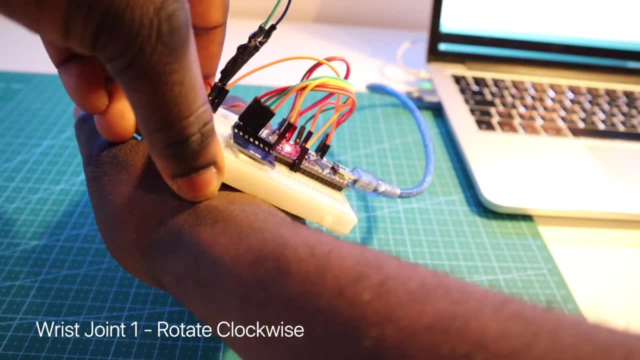 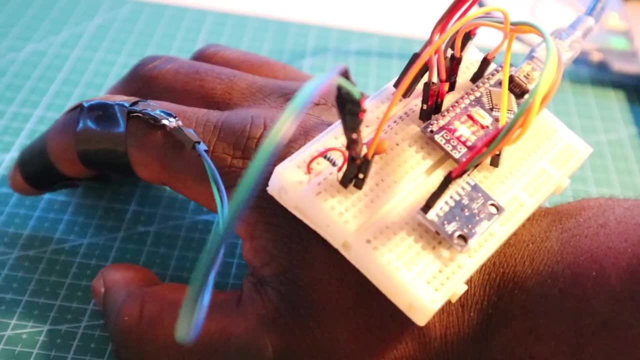 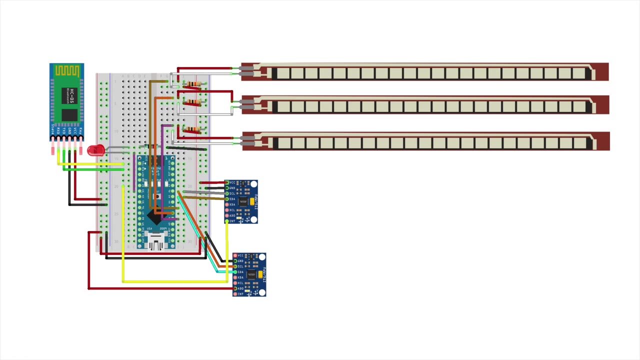 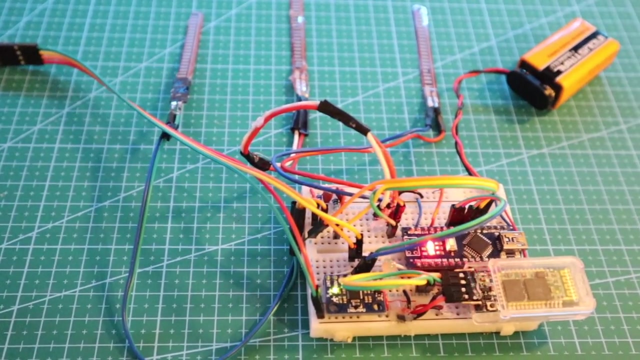 rotating the gripper counterclockwise or clockwise, as well as up and down. Now this idea will form the basis of the 3D glove, and for this I pretty much added two extra flex sensors and another accelerometer, which can be powered from a 9-volt battery Adding additional sensors. this is what the electronics 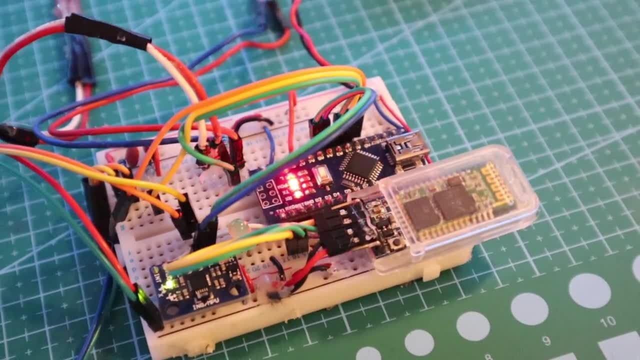 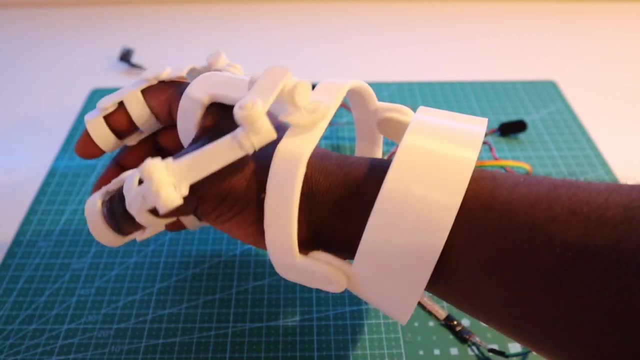 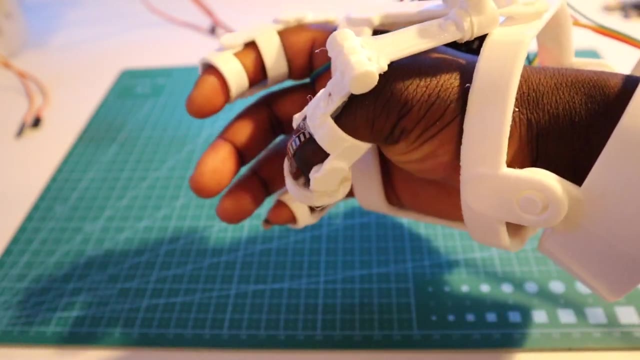 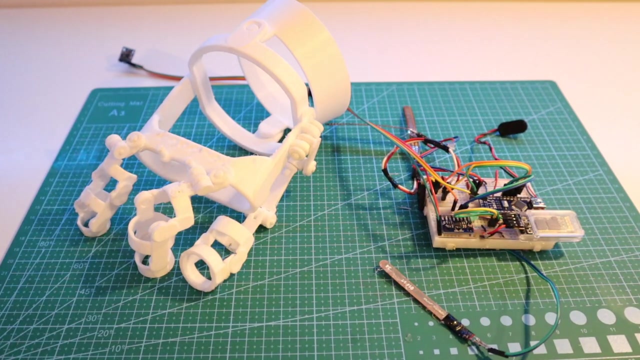 looks like, with a Bluetooth module to communicate with the robotic arm. Now the next step is attaching the electronics to the robotic glove, going from this to this, where we can bend the flex sensors which are mapped to each finger, and the most important thing about the assembly- 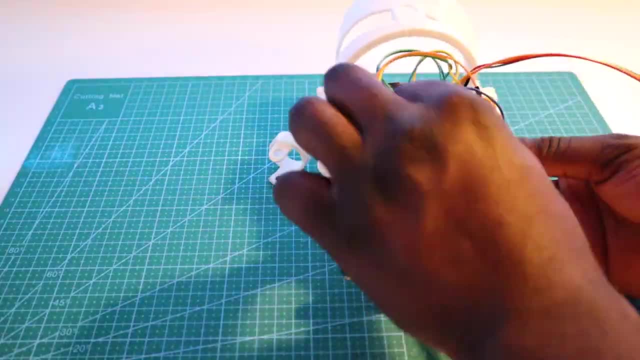 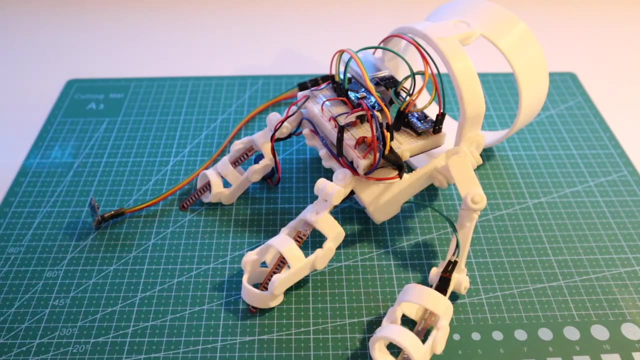 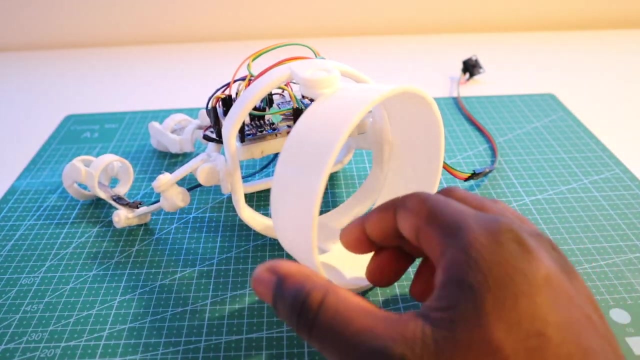 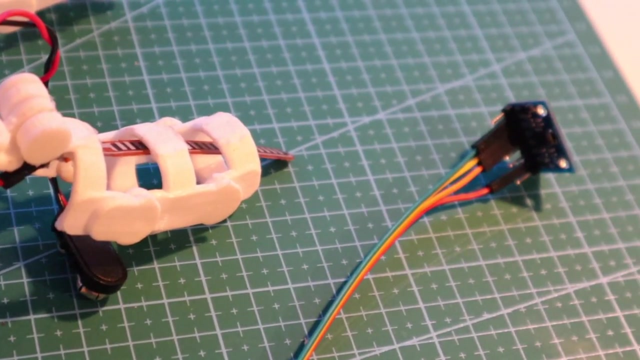 is securing all sensors in place, and to do this we can use hot glue, and this is how we're going to wear the glove. Given that all sensors are now being added, we can now go into more detail on how every flex sensor maps onto the arm. You can see how each sensor 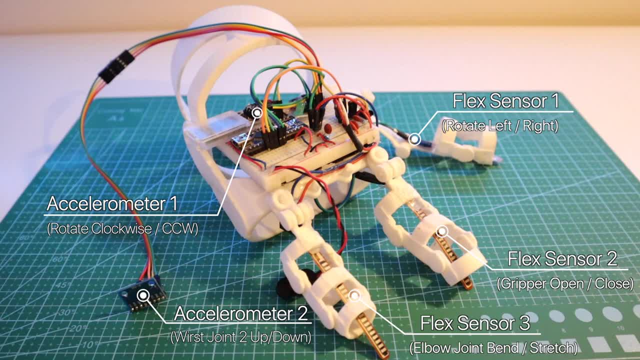 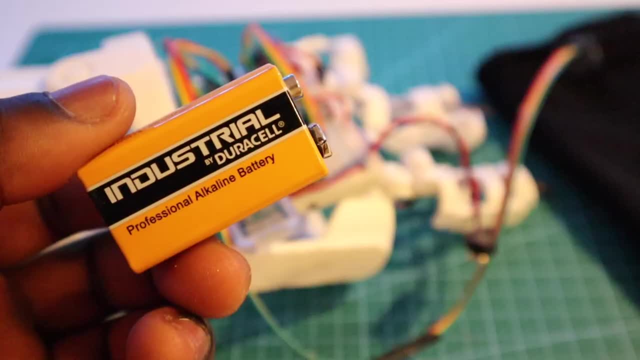 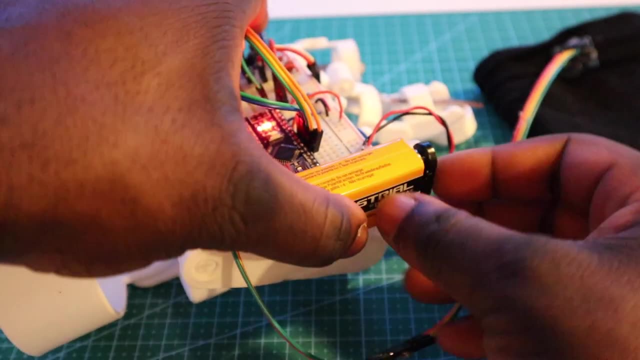 represents a servo on the robotic arm. Now, this is optional, but you can even add the second accelerometer to an armband, as well as a 9-volt battery, which was added to make the robotic glove portable. and this is pretty much the robotic arm prototype on a breadboard. 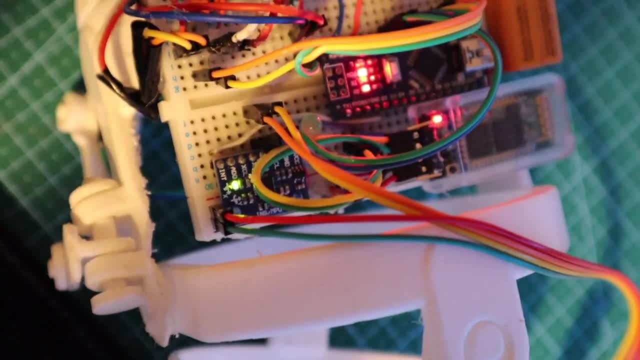 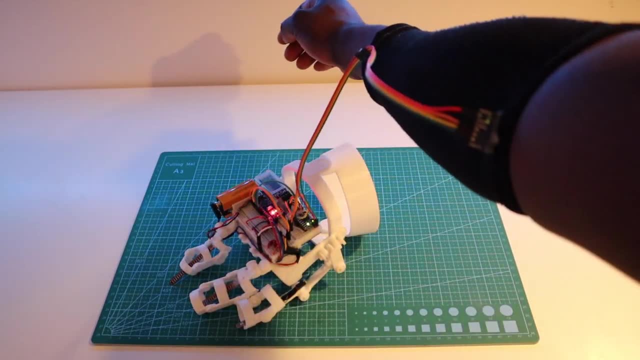 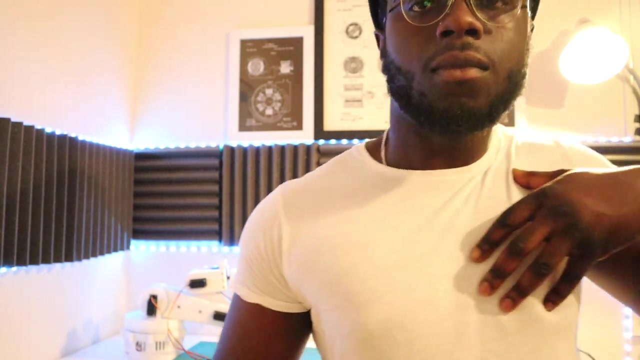 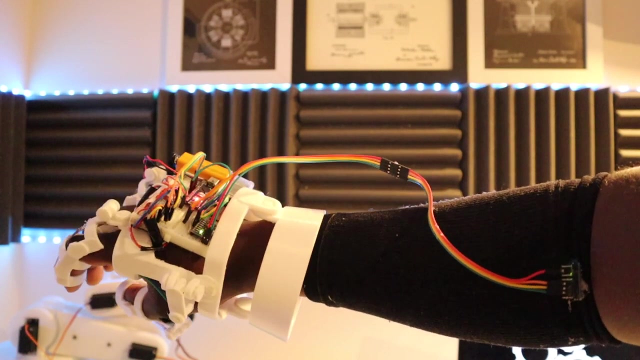 We'll see how we can make this more advanced. now, believe it or not, the robotic glove required me to isolate some of my joint movements to not trigger any false positives, and this is where body isolation became useful. Here it is all assembled and, finally, the build. this is what each part does. 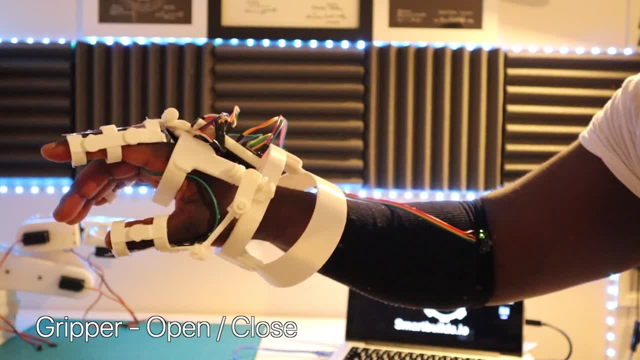 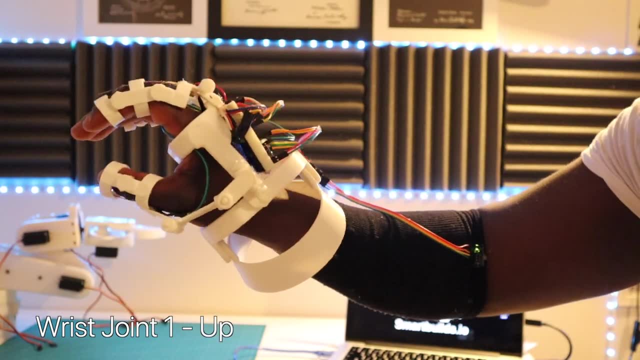 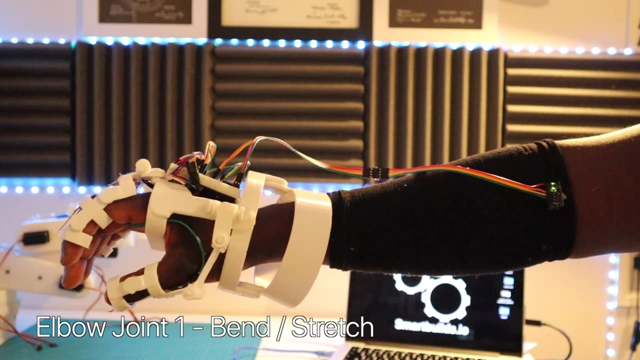 So opening and closing the robotic claw can be done by moving our index finger up or down and rotate, and counterclockwise or clockwise will move the grip ahead as well as up and down, and we can rotate the whole robotic arm left or right or bend or stretch to move the robotic elbow. now, that is the 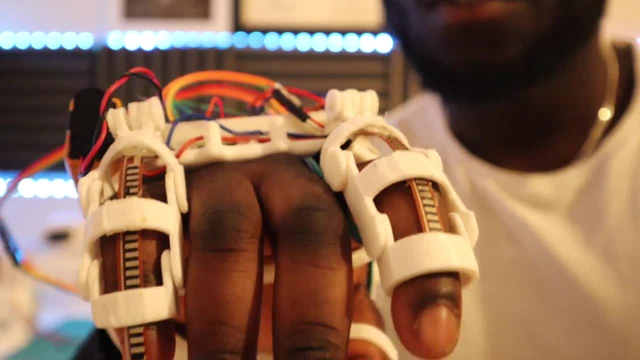 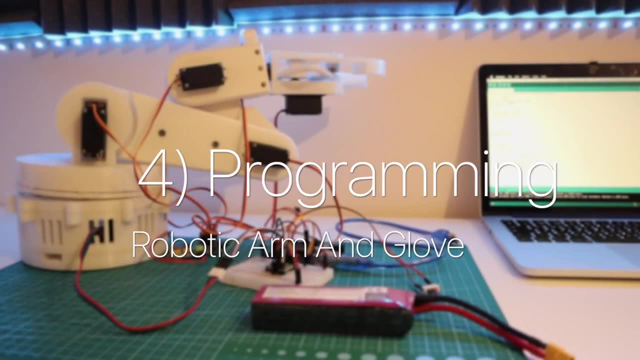 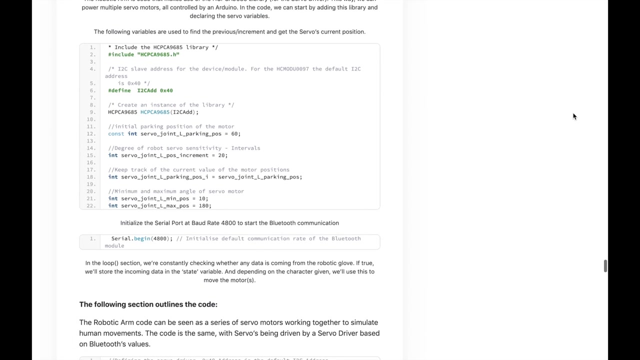 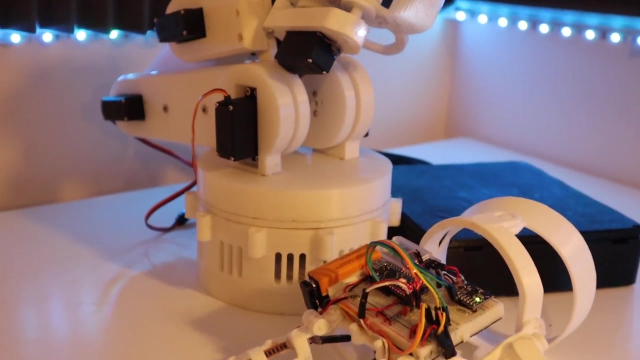 robotic glove and arm. pretty much done. Now let's get back to the code to see how the programming really works. Now the programming part is explained in more detail on the article in the description below, but it's still important to go over the key parts. Ideally, there are two main codes: one for the robot arm and the 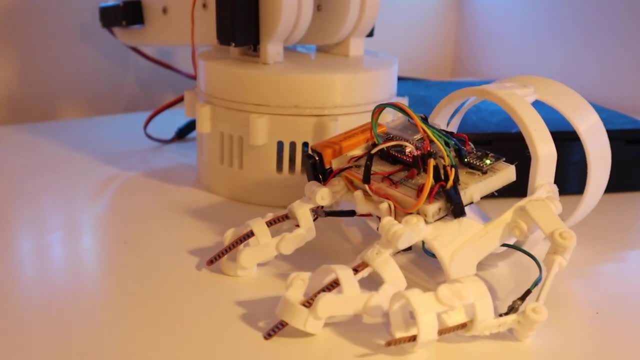 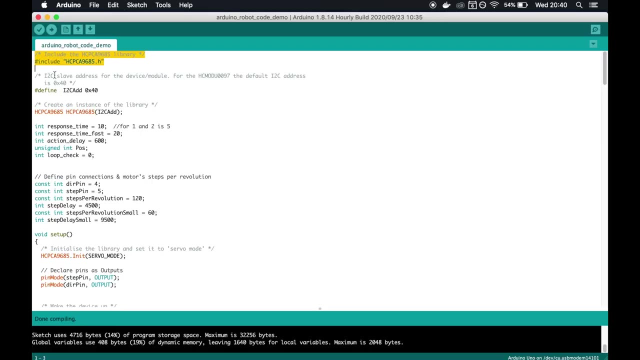 other for the glove being the controller in this case. So let's start off with the robot arm and see how this will be programmed. To start off, the robot arm includes the server driver library being the PC9685. this way, we can power multiple servos, all controlled by an Arduino. This will 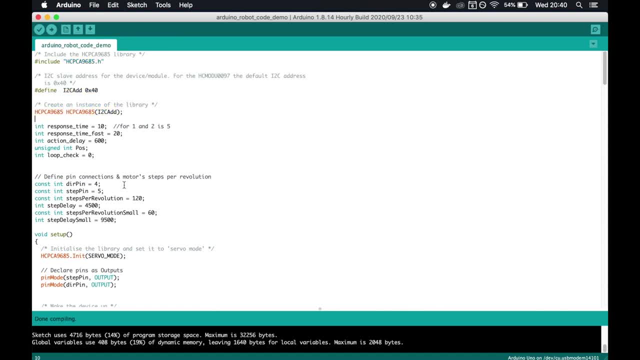 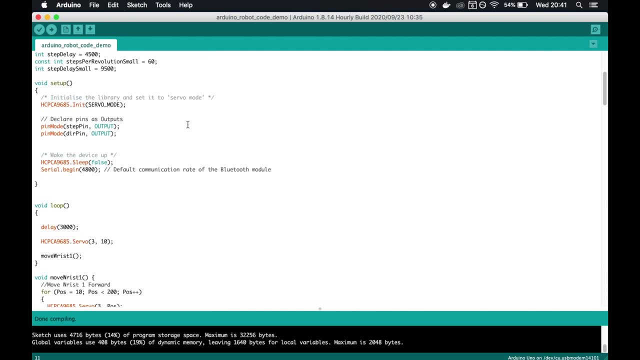 be used rather than using the standard server dot write function. The following here declares and initializes the variables for the stepper motor and in the setup we can declare the pins used for the server and stepper motor In the loop section. I've added a delay of three seconds on startup, so the robot 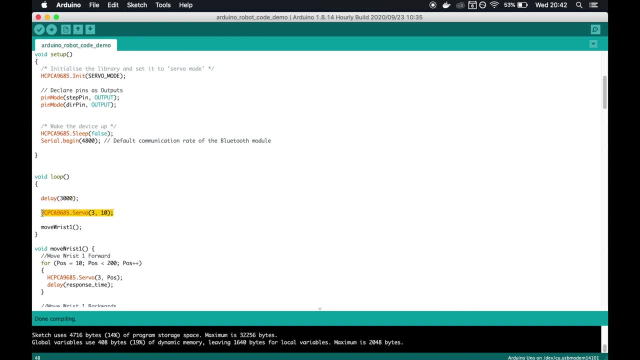 doesn't jump at you straight away. Now, the way we control the server motors is by using the library name dot servo. this takes two parameters: the position of the server plugged on the driver, starting from zero, and the position we'll like to move it. In this case, we'll be moving the server on channel 2.. 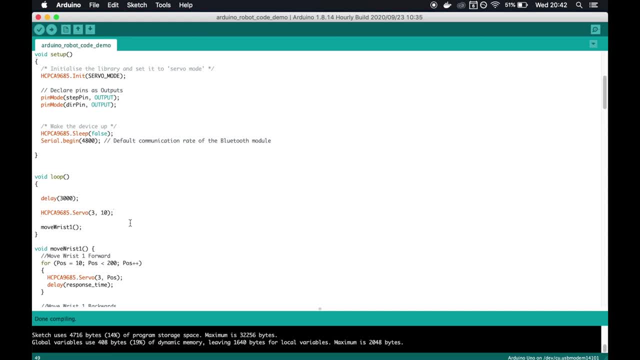 In this case we'll be moving the server on channel 2. to the relative position of 10.. Now, with that theory we can pretty much make a function that can move the wrist part of the robotic arm, as seen here, and from there you can make other functions like opening, closing the claw and making the 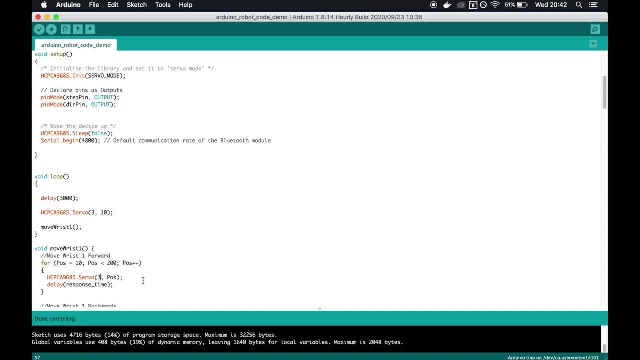 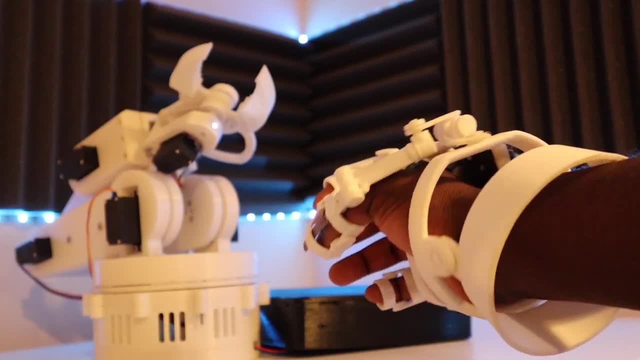 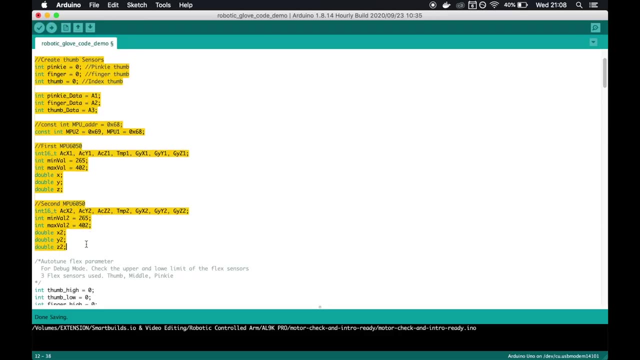 robot stand. and that's pretty much it for the robotic arm alone. but if you would like to take one step further and control the robotic arm with the robot glove, here's the code. Now for the robotic glove. as mentioned, we have three flex sensors and two accelerometers, and these are 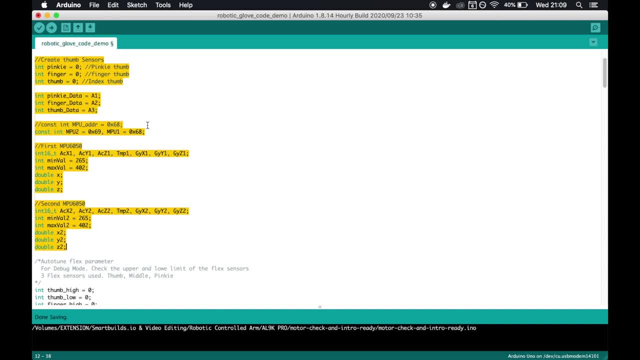 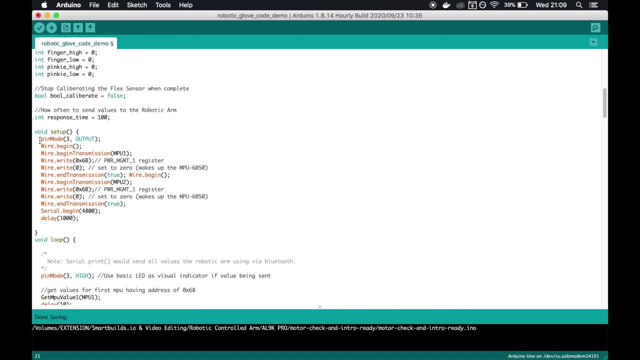 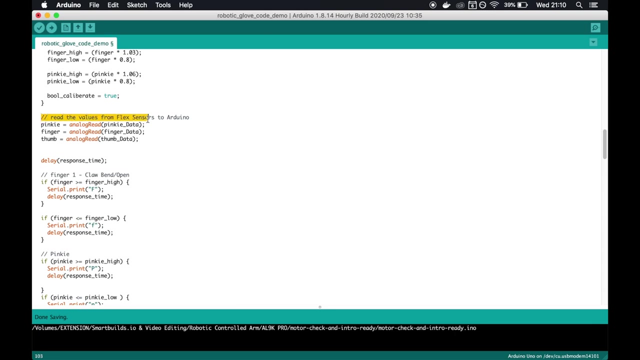 initialized here. We'll first off declare the three sensors on the thumb, pinky and middle, as well as the accelerators In the setup. we'll begin the transmission of the sensors, including the Bluetooth serial communication at the baud rate of 4800.. Now in the loop section we'll read the values of the flex sensors to the Arduino and 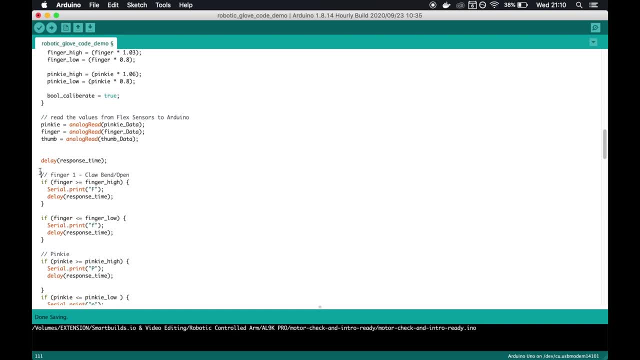 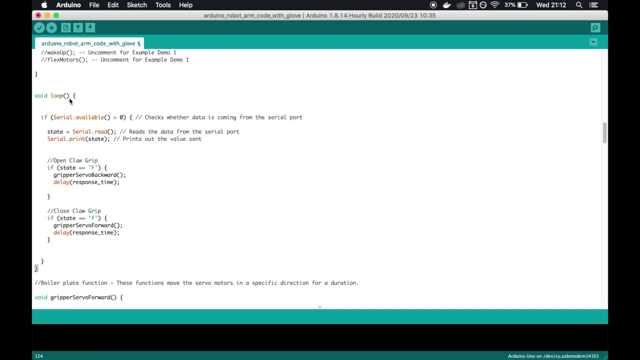 based on the previous theory, when the value of the flex sensor bends exceeds the threshold, this is when we'll send the character f and this value is what will be sent through Bluetooth to the robotic arm and if we go back to the robotic arm code we can create. 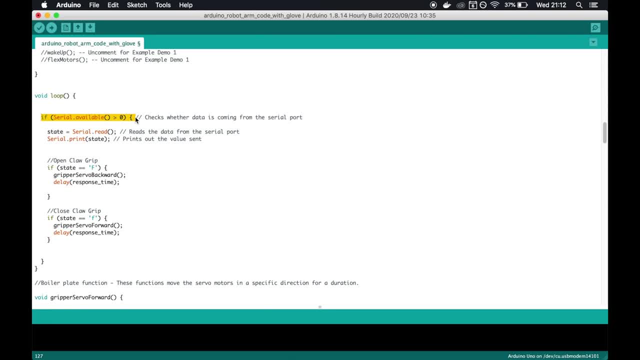 a function that listens on the baud rate of 4800.. Now in the loop section we'll read the values of the flex sensors to the arduino and based with the bluetooth module and if it receives the character f, this would then call on the gripper server backward function, which will move the server, and this is an indefinite loop. 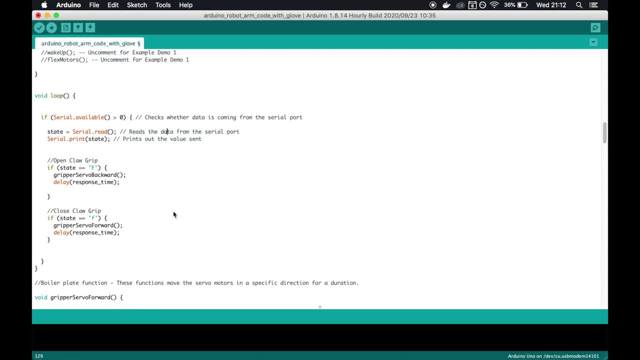 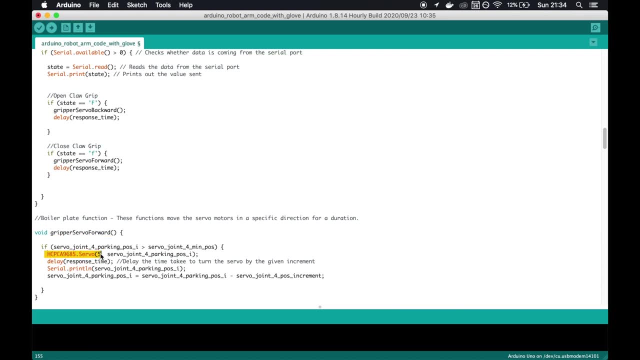 always waiting for communication from the glove to the robotic arm, and we have an example function here whereby we're moving the server on the fifth channel of the server driver, and we can create as many functions here, and that's pretty much it for the programming. it's now time to put everything. 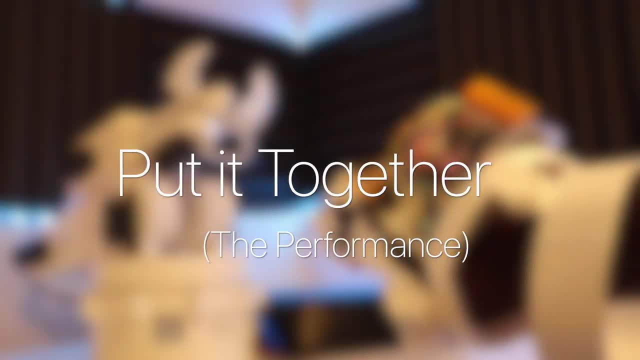 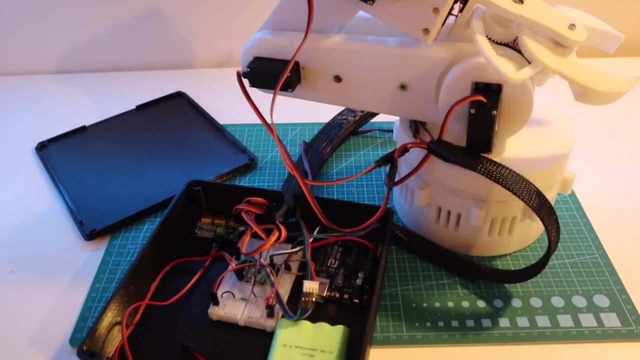 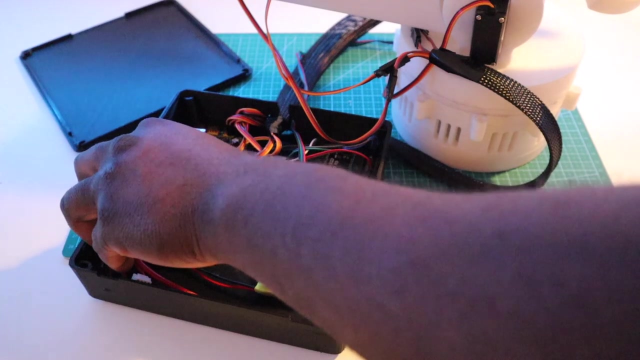 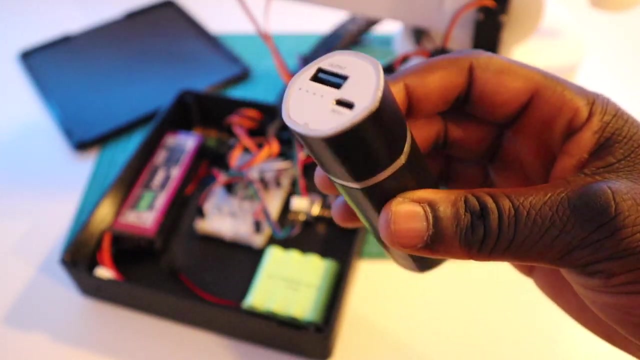 all together. now putting it together, a 3d printed enclosure was used to encase the circuitry of the robotic arm, as well as some braided cables for protection, and now we can finally place all our circuitry into the enclosure. you and we can use a simple power bank to power the arduino. 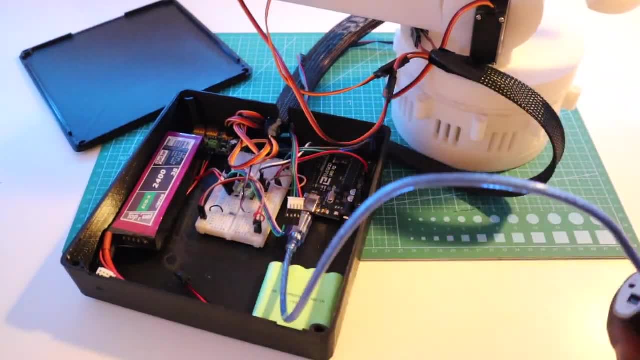 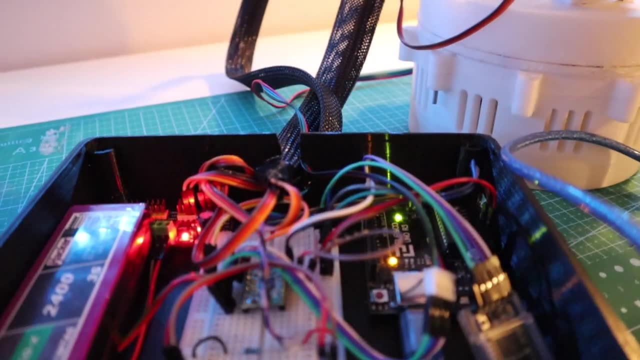 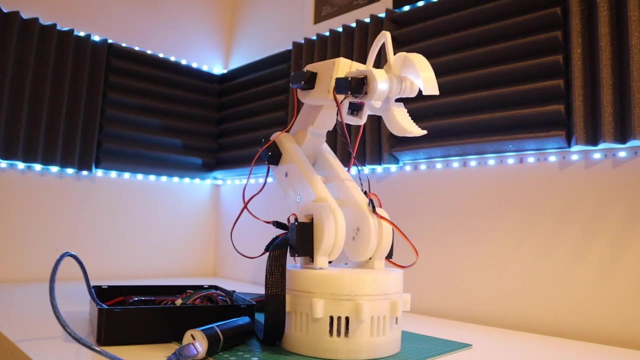 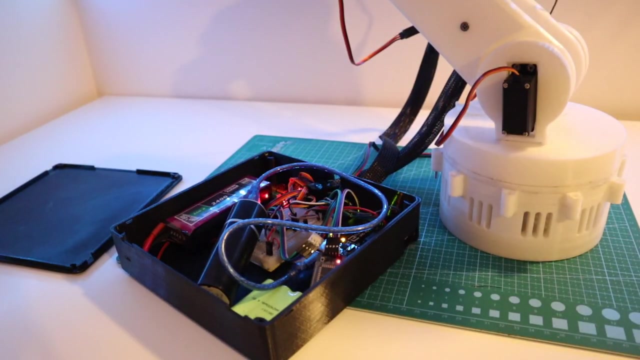 and this is it. this is absolutely everything you'll need in terms of hardware to work with this robotic arm prototype. now let's test it out. in this example, we have the robotic arm waking up and we can just pretty much close the enclosure, which has a snap button, and we can just close the enclosure. 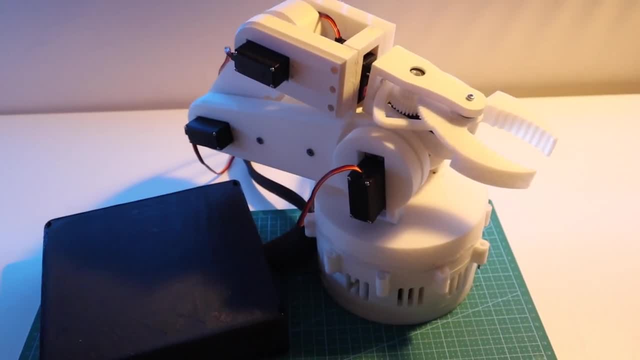 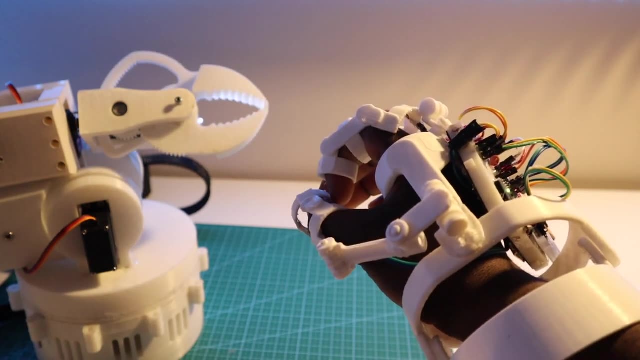 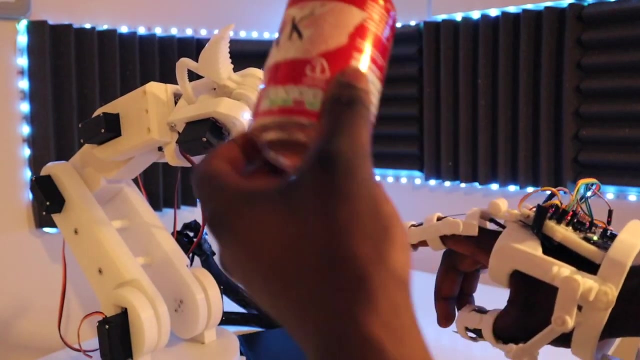 on lid and now it's programmed. it's now time to test it out. and if we bend the flex sensor, the value changes and this is sent to the robotic arm. so how does the robot arm respond to hand gestures? well, the prototype is pretty responsive and works. however, the robot glove is pretty sensitive. 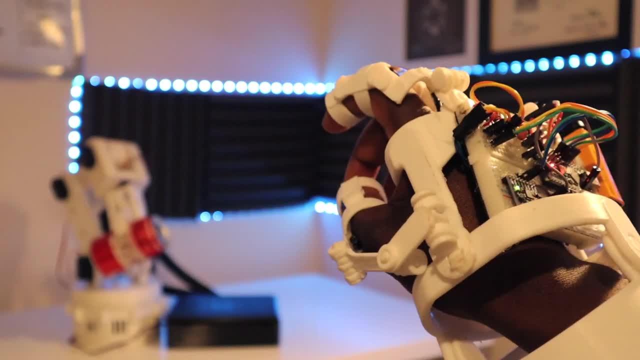 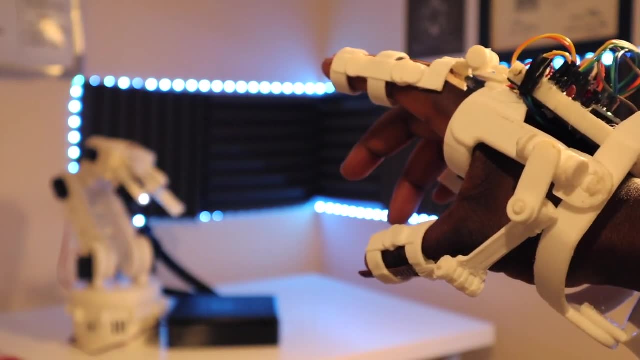 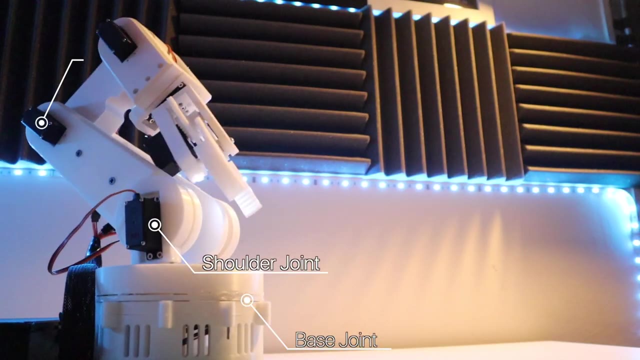 as it had quite a few sensors plus. it was a bit of a learning curve to control the robot without altering other parts of the arm, but the good thing is these are programming related and improving the code should improve the accuracy and the fluidity of the arm. we'll revise this prototype sometime in.